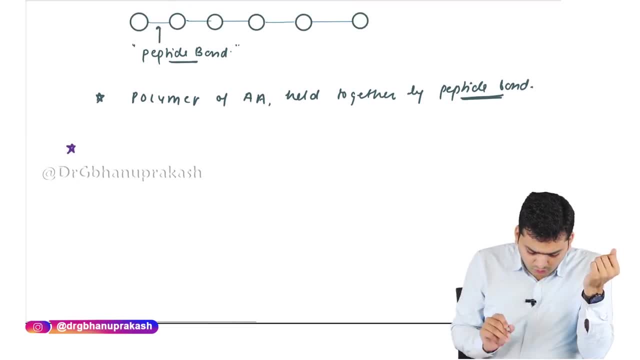 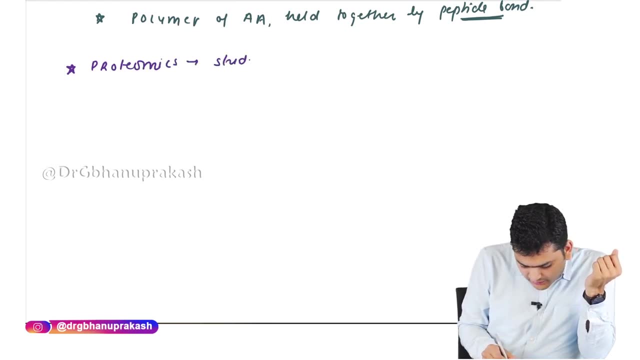 inside the biological environment is referred as proteomics. So what is proteomics is? Proteomics is the study of protein structure and function. structure and function inside the biological environment. inside biological environment, that is referred as proteomics. Now, once we are clear with this definition of protein, 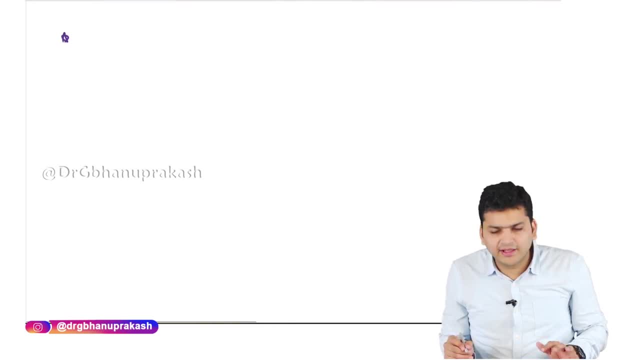 protein and proteomics. Now let's see, we know that a cell is continuously producing different types of protein. Say, for example, let's say: this is a cell and it is producing different types of protein and making with different shapes. For example, this is the. 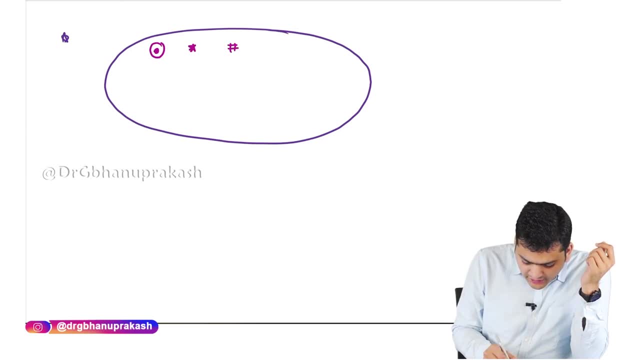 protein A, protein B, C and so on. We can have different types of protein A cell continuously producing different types of protein. So how these proteins will be differentiated from one another. there is an organelle that is with the name of golgi body. what golgi body will do is 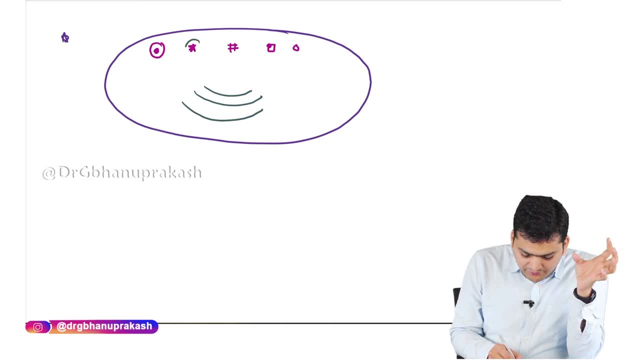 golgi body will make recycles and in these recycles these different, different proteins will be packed in different, different recycles. so i can say: this is a sorting of protein. this is a kind of sorting of protein that is occurring and they ask that this sorting of protein occurs with the help of 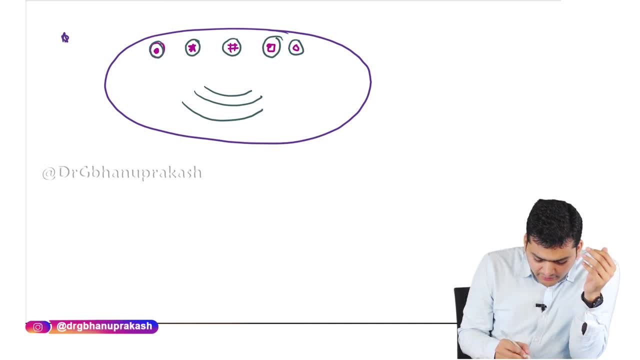 which organelle? the answer will be golgi body. so let's write down the statement that sorting of protein, sorting of protein, is done by golgi body, sorting of protein is done by golgi body. this is one thing. once we are clear with this structure, once we are clear with the basic definition of 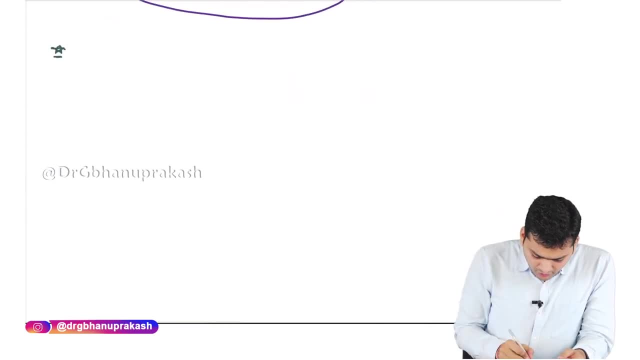 now we'll see the classification of protein. so so now we'll start with the classification of protein, protein. whenever we want to classify anything, first we need to understand that on what ground, on what basis, we are doing this classification. so the first classification that we are going: 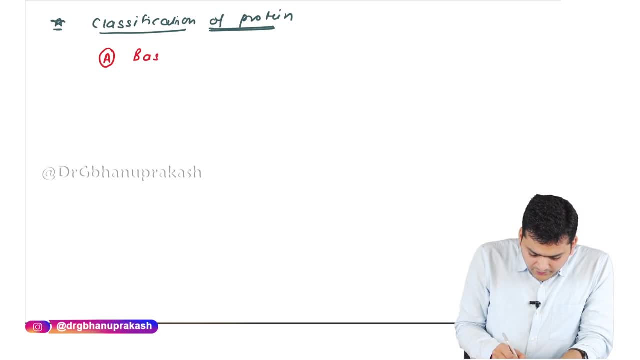 to discuss of the protein is based on, based on nutritional value, based on the nutritional value of the protein. based on the nutritional value. now, what is the meaning of nutritional value? see, we know that we have total 22 types of amino acid. out of 22, we have 9 essential. 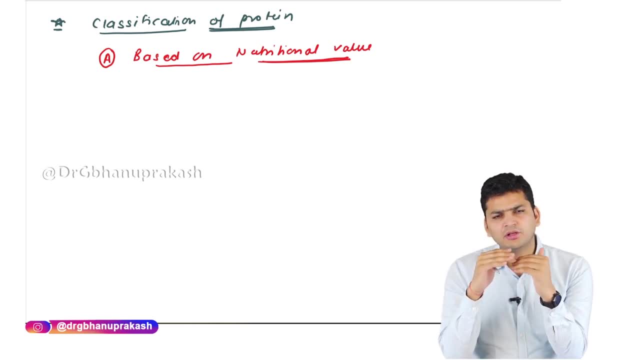 amino acid. so these 9 essential amino acid has to be taken in the diet because the body cannot synthesize them endogenously. so what i can say is that, based on nutritional value, i can say that there are some protein source which contain all the 9 essential amino acid. 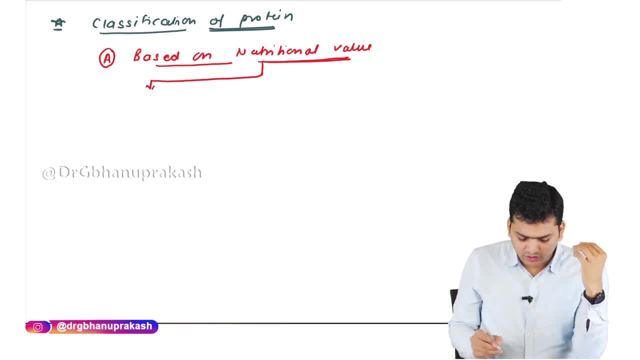 if there is any protein source which contain all the 9 essential amino acid, that is called as complete protein. complete protein in a sense that if you are eating that particular protein source, there is no other requirement to eat any other protein source, because that will suffice all the essential. 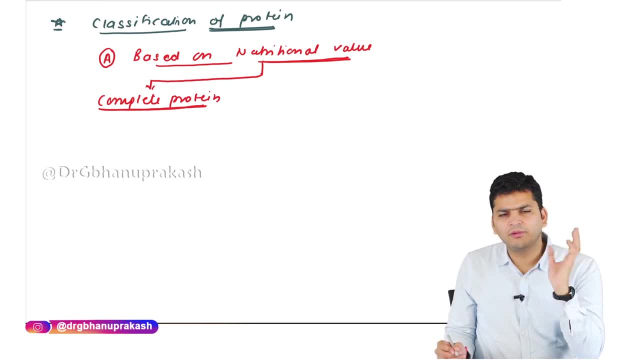 amino acid you are taking. the rest of the amino acid will be made by the body itself. so i can say what is complete protein is basically contains all essential amino acid, contain all essential amino acid, and the example of such complete protein is casein. casein is: 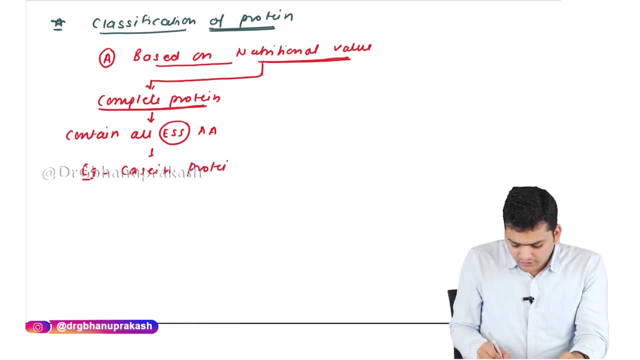 the protein that is found in meat, casein, protein of milk. so if we are taking casein in our diet, then the all the essential amino acid we are taking primarily and from that the other non-essential, semi-essential will be synthesized. so this is the complete protein. complete protein is also referred. 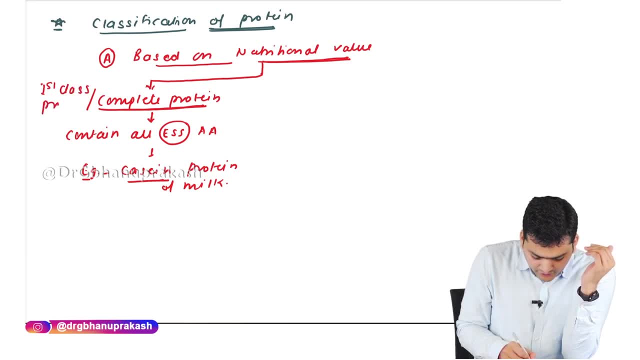 as first class protein. also referred as first class protein, then the- the second classification is the second subcategory- is that is called as incomplete protein. incomplete protein, now, what is incomplete protein is basically, if we are taking a protein source which lake one essential amino acid, if there is only eight essential are present. 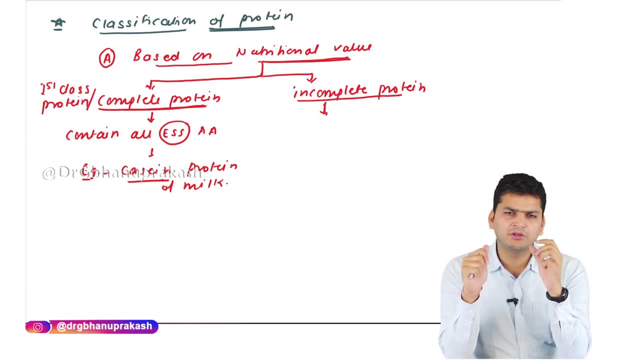 and one essential is missing because total nine essential. we have nine essential amino acid. out of that, only eight are present. one is missing. such protein source are labeled as incomplete protein. so incomplete protein means contains eight essential amino acid, or i can say lake one essential amino acid and one essential amino acid, so incomplete. 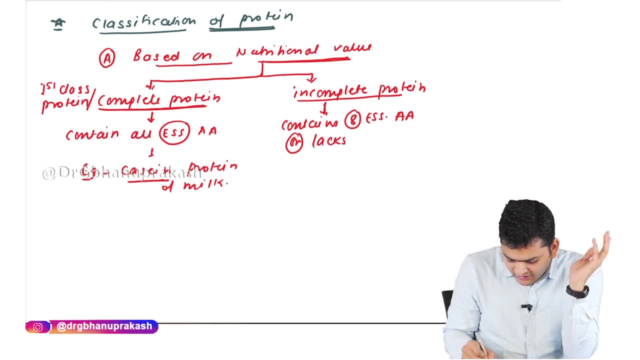 protein means contains eight essential amino acid, or i can say lake one essential amino acid and one essential amino acid. so incomplete protein means contains eight essential amino acid or i can say lakes one essential amino acid. the example is pulses. pulses are deficit of methionine. pulses are deficit of methionine between is essential amino acid in the same. 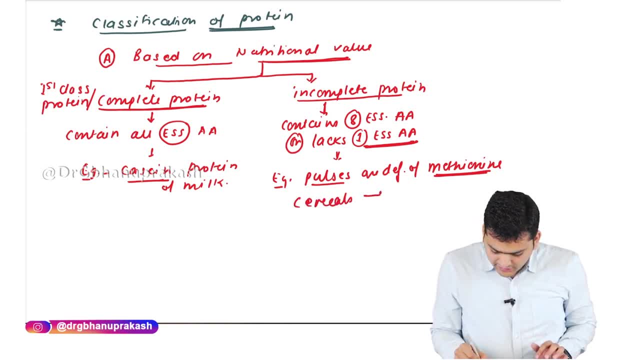 way we can add: uh, cereals. cereals are deficit of lysine, so pulses, pulse Гос shrine life, so deathsleri38vin ə. så Methionine cereals, lysine. So they are deficit of one particular essential amino acid, So they 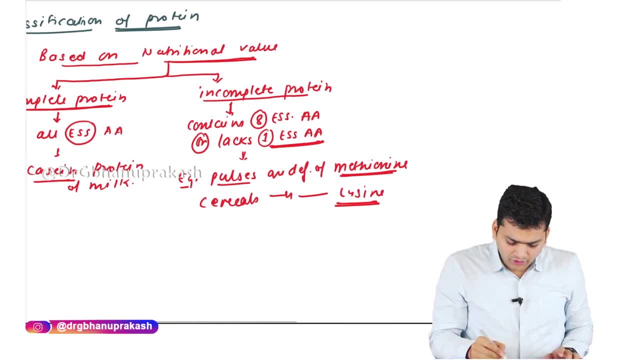 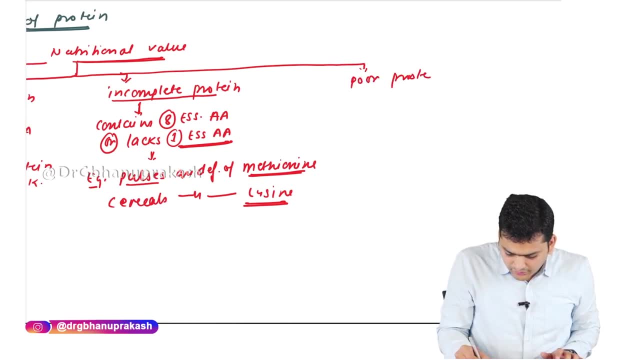 are the incomplete protein sources. Now there is one more category, and that is referred as the poor protein. Poor protein, Poor protein means more than one essential is missing: Means, two or more than two essentials are missing. Two or more than two essential amino acid are missing. 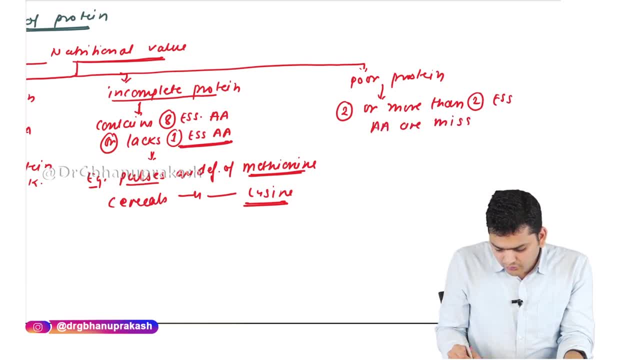 If two or more than two essential amino acid are missing, that is called as poor protein. The example is: the example is the Zene protein, Zene protein found in corn. So this Zene protein, which is found in corn, it is particularly deficit of. 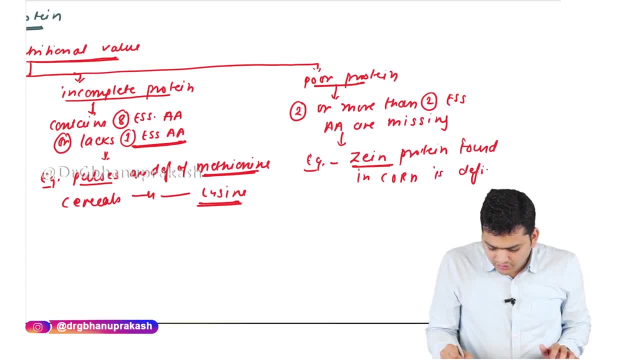 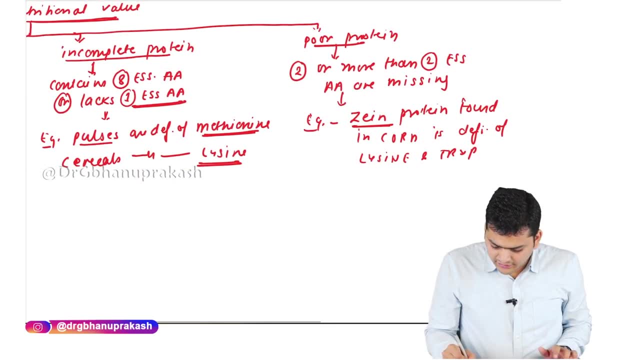 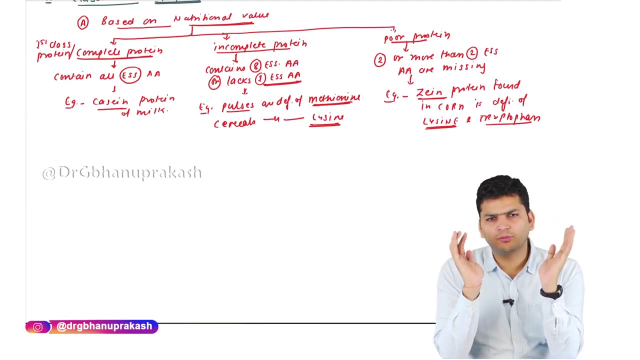 is deficit of is having deficiency of lysine and tryptophan. Lysine and tryptophan Is deficit of lysine and tryptophan. To summarize, I can say that there are three categories of protein we have: Complete, incomplete and poor. Complete means all the nine. 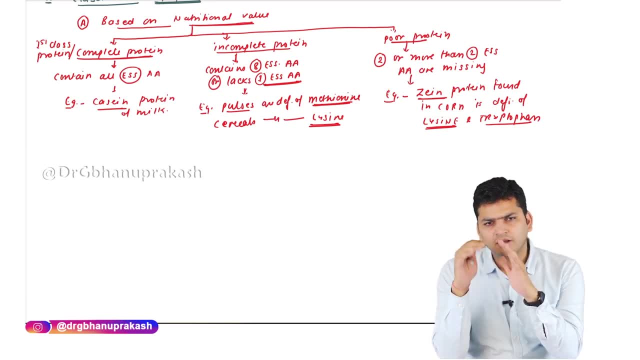 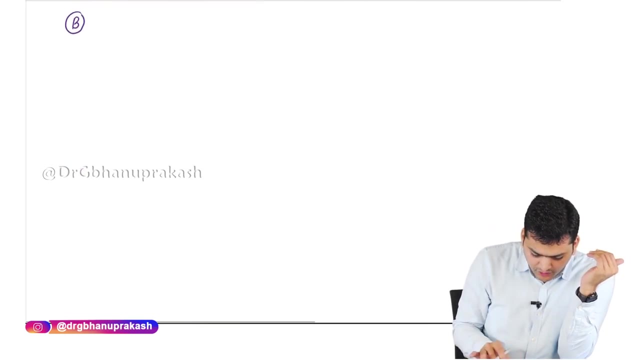 essentials are there. Incomplete means one essential is missing and poor means there is more than one essential Means, maybe two, or maybe more than two. they are missing. So this is the first classification that is based on the nutritional requirement or the nutritional value. Let's see the second classification of the protein, That is basically: 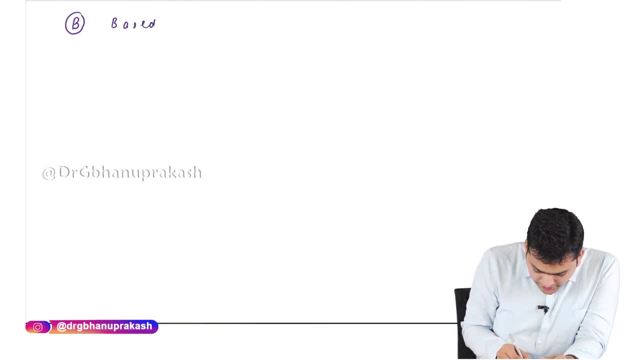 basically based on the structure of the protein, Based on structure of protein. Now, when we classify the protein based on the structure, the sub categories, you may be aware of that. the sub category is based on the structure. They are the primary structure, the secondary 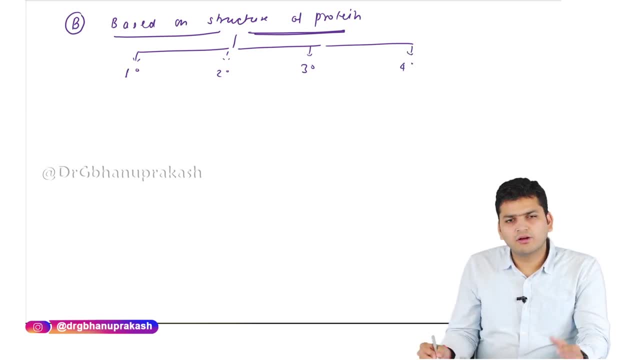 structure, the tertiary structure and the quaternary structure. So we are going to discuss them in detail: primary. what is secondary, and so on. so let's starting with the first one, that is, the primary structure of the protein, primary structure of the protein. so to understand these primary, 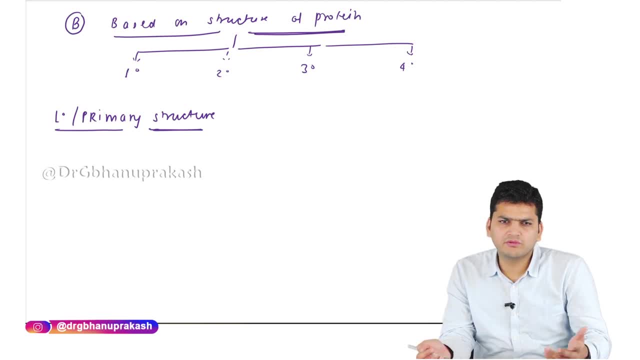 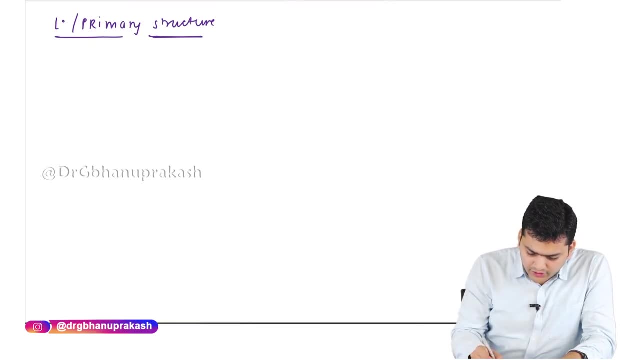 secondary, tertiary, quaternary. first, we'll make the structures and from that structure we'll be trying to derive the definition. so, primary structure of protein. when it comes to the primary structure of protein, what we are going to notice that in the primary structure of protein there are amino acids. say, for example: these are the amino acid, this is the. 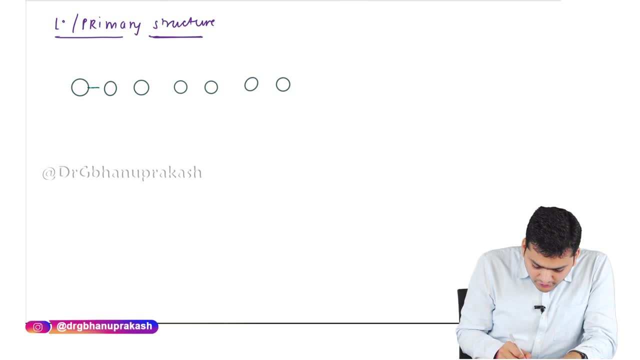 polymer of amino acid we are making and the only bond which is going to be there in between, the only bond which is going to be there in between, is the peptide bond. there is no other bond than the peptide. so i can say: here is your peptide bond and these are the amino 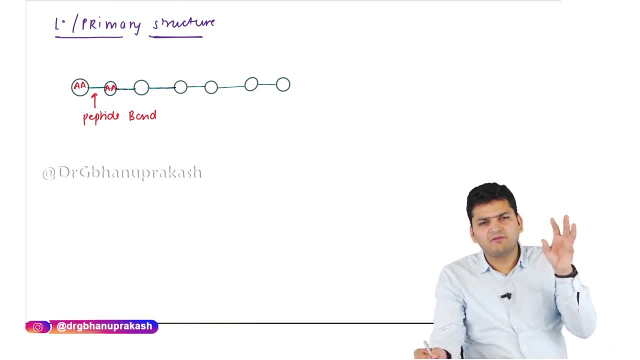 acids. so basically, there is a chain of amino acid which is held together by peptide bond and that is called as the primary structure. this is the simplest structure possible. there is no other than peptide bond. there is no bond other than peptide. so primary structure is is basically a polymer of amino acid or a. 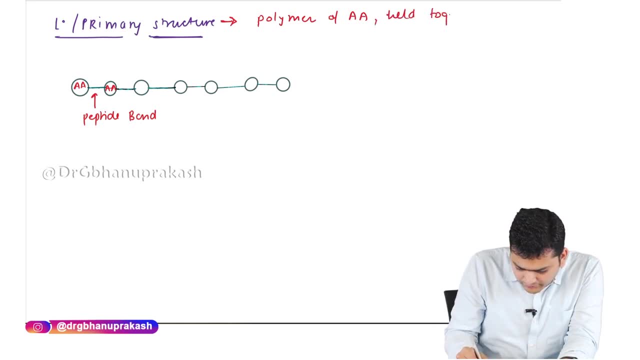 chain of amino acid held together by peptide, held together by peptide. now, the point to be remembered is that the peptide bond is a covalent bond and the covalent bond is a peptide is a very strong bond, is a very strong one. so peptide bond is a strong bond and hence, 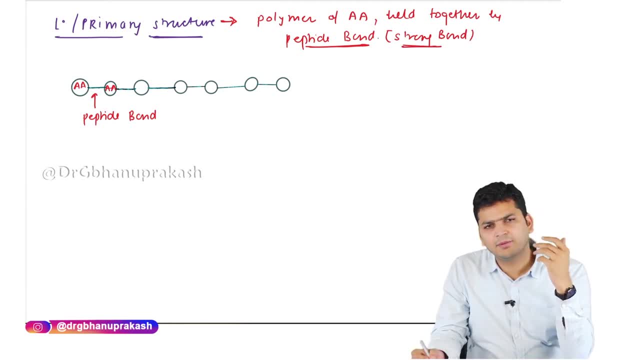 we can say, because it is a strong bond. so, and we can say that the primary structure of it is going to be the strongest structure among all these four- primary, secondary, tertiary, quaternary- because it contains only the strong in, that is, the peptide. 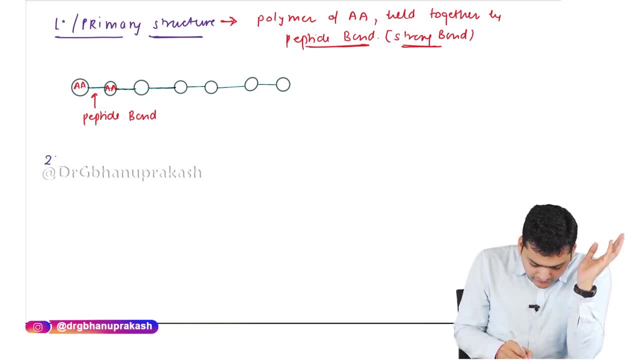 now coming to the second structure, 2. клиtens3, our second structure, 解釋. let's first understand the definition of the secondary structure. to understand the definition again, i am drawing a diagram. from the diagram we'll try to derive the definition. so, for example, let's say: this is the amino acid, the amino acid. 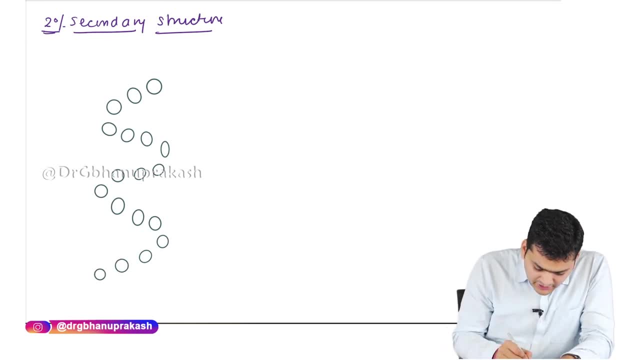 so i have made a chain of amino acid and this chain of amino acid- again the bond that is going to be there in between is the peptide bond. so i have made a chain of amino acid and there is a peptide bond in between. so till now it is more or less like the primary structure. now what i do is: 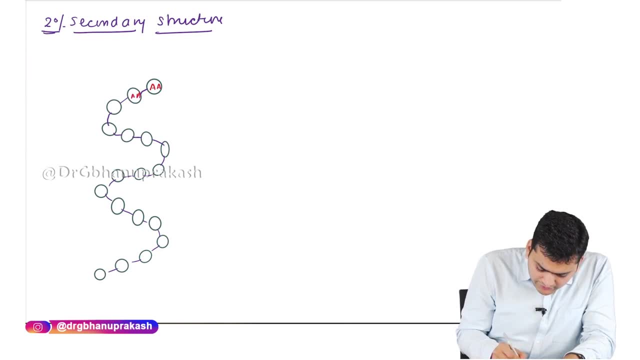 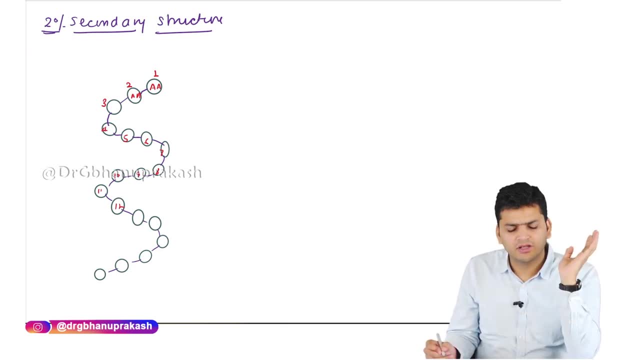 non-peptide relationship between the amino acid which are in the linear sequence means, for example, the amino acid number two, amino acid number two and the amino acid number six. they are in the linear sequence. they are linear sequence. they are three amino acid apart from one another. 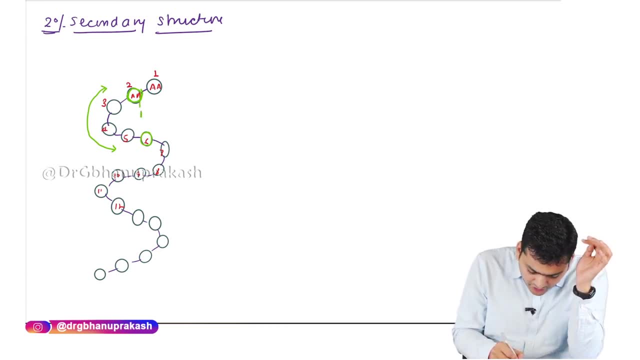 now what i do is i make a non-peptide bond in between these two amino acid non-peptide bond. then again i make a non-peptide bond between, let's say, from the amino acid number five and ten- again they are in the linear sequence- three, four amino. 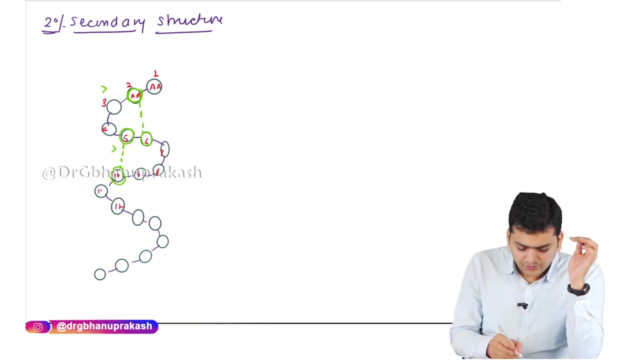 acid apart. so it's making a non-peptide bond in between. so if we make the non-peptide relationship in between the amino acid which are in the linear sequence like this, then this relationship, this structure, is going to be referred as the second structure. so this green color bond which i made, 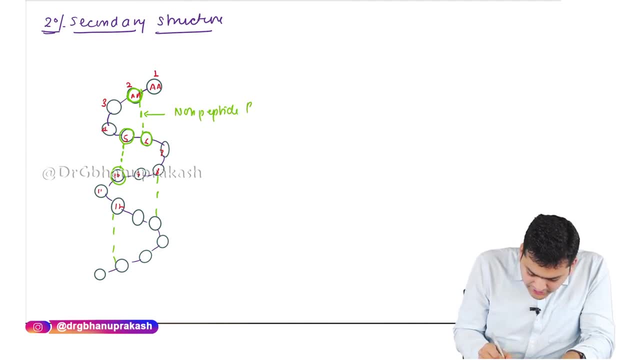 is the non-peptide bond. in the primary structure there is only one type of bond that was there was the peptide bond. in the second structure we have the peptide as well as the non-peptide bond. so the second structure i can say is: if i derive the definition from the uh, from the diagram, if we derive the 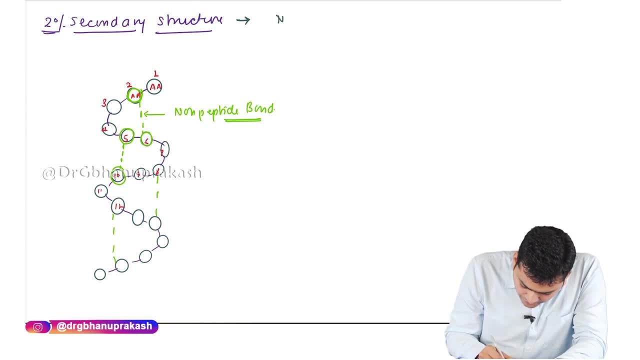 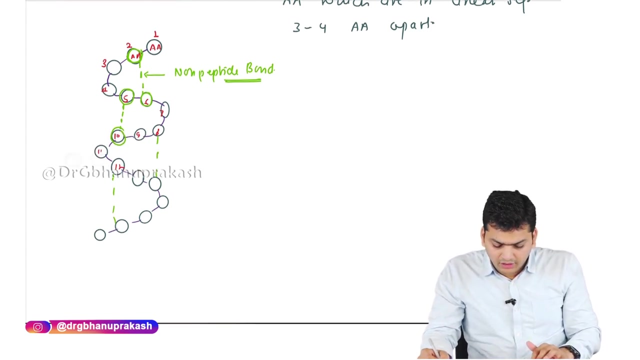 definition. what i can say is there is non-peptide relationship between the amino acid which are in linear sequence, three, four amino acid apart. we are making a non-peptide relationship between the amino acid which are in the linear sequence, three, four amino acid apart. now, once i'm saying it is non-peptide. 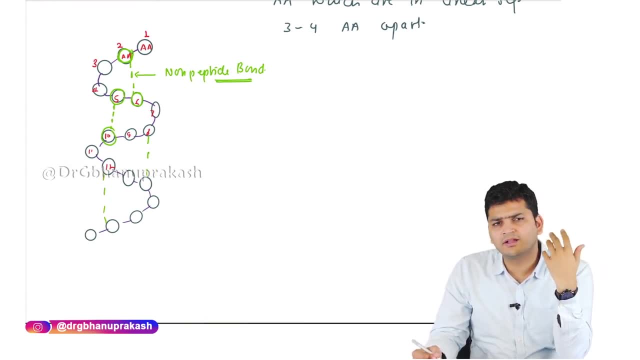 bond. so which type of non-peptide bond, which type of, or what are the examples of non-peptide bond we have? so let's write down the examples of the non-peptide bond or the non-peptide relationship. the non-peptide mode, the most commonly the non-peptide bond that we are going to see is 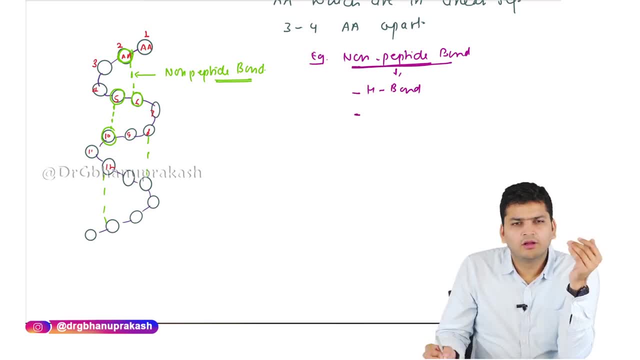 the hydrogen bond. the hydrogen one, then other than hydrogen bond it can be, such as the wonderwall one. it can be electrostatic bond, it can be hydrophobic bond. so the point is that it should be. it should not be a peptide bond. it should be other than peptide. it should be other than peptide bond. that has to be. 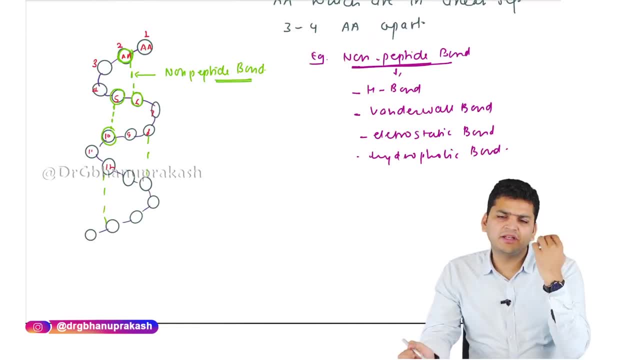 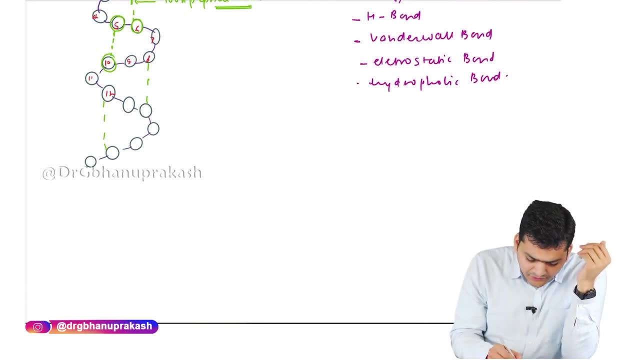 there in a secondary structure. now, once this, uh, the basic diagram is clear that how the secondary structure is made, how we are going to make the known peptide relationship, now we'll see the, the subtypes of the peptide. now we are going to see the subtypes of the secondary structure. subtypes- secondary structure. so, when it comes to the subtype of the secondary structure, what we can see is the subtypes are alpha, helix, beta pleated, sheet turn and bands loops. so these are the types of secondary structure that we have: alpha helix, beta pleated sheet turn, band- and so let's discuss them one by one. 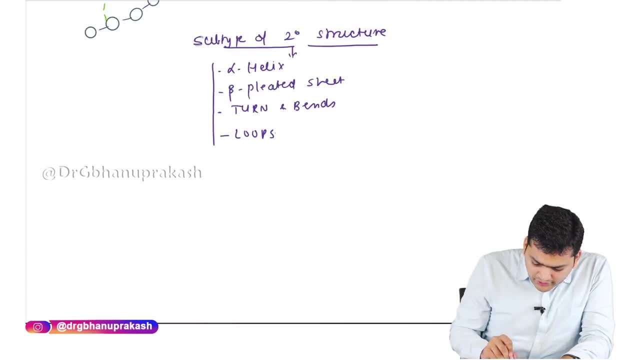 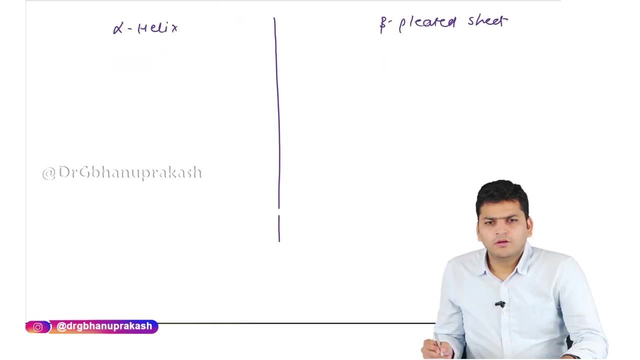 first of all, we'll start with the alpha helix and the beta pleated sheet. so we'll try to make a differentiating table in between. we'll try to make a differentiating table in between the alpha helix and the beta pleated sheet. alpha helix and the beta pleated sheet. now let's first make the structure of the alpha helix. 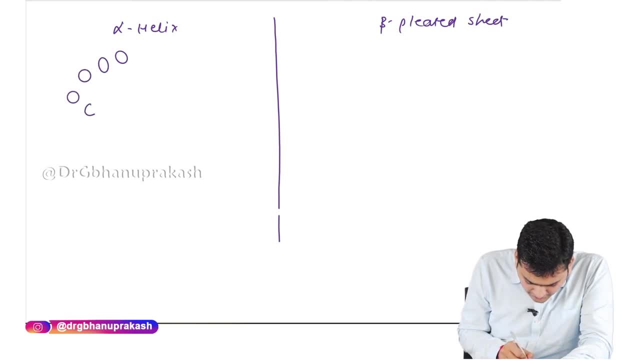 in the alpha helix we are going to have the chain of amino acid in a helical shape manner. there is only one chain and the bond. firstly we are making the peptide bond and in this single chain now we are going to make the non-peptide relationship also. 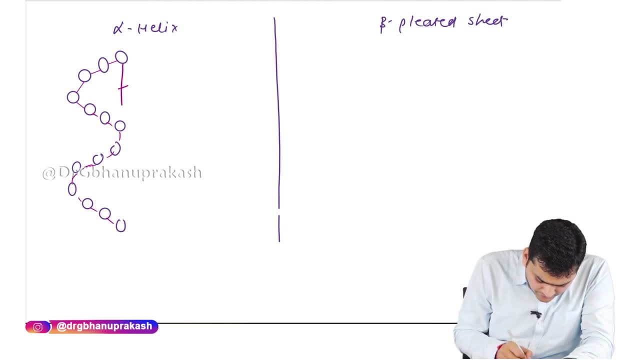 so let's say these are the non-peptide bonds. so these are the non-peptide bonds. the green color ones are the non-peptide one. when it comes to the beta pleated sheet, there will be more than one chain of amino acid. so, for example, this is the first chain. 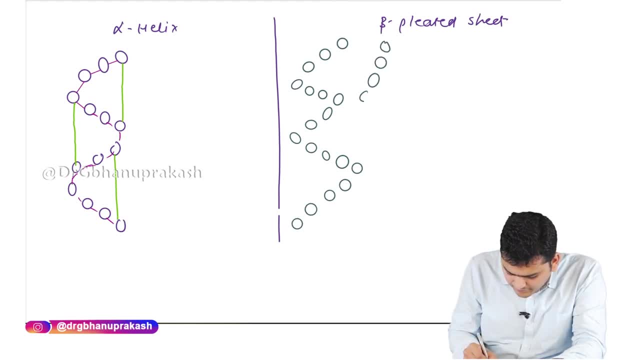 this is the second chain. so basically there will be more than one chain and between the amino acid, the first is going to be the peptide bond. so this is the first polypeptide chain, this is the second polypeptide chain and now we are going to make the non-peptide relationship. so, for example, let's say so now: 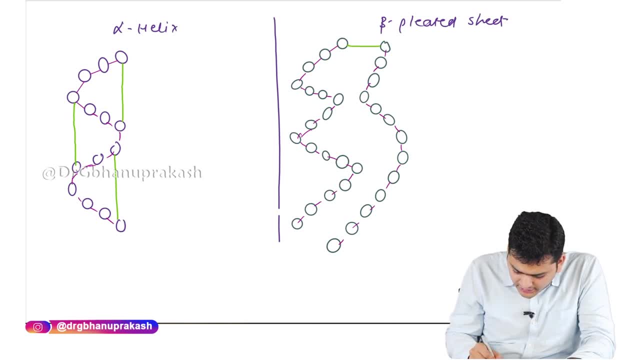 we are going to make the non-peptide bond say, for example, let's say these are the non-peptide bonds in between the chains. so what you can see is in the alpha helix there is only one chain that is there and it is looking like a helical shape structure, whereas in the beta pleated sheet 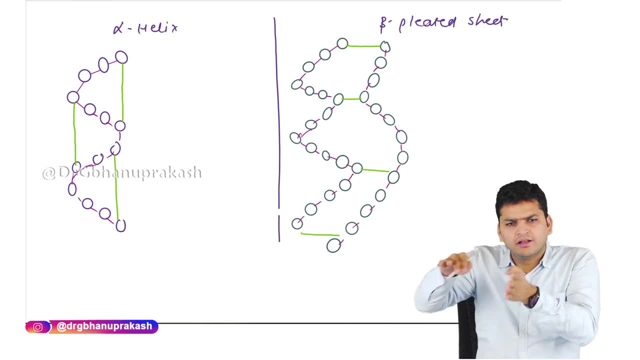 there is more than one chain and if you see the structure, it is looking like this, like a zigzag pattern. so if we make the difference between these two types of secondary structure- the alpha helix and the beta pleated sheet- the first difference that we can figure out is that the alpha helix 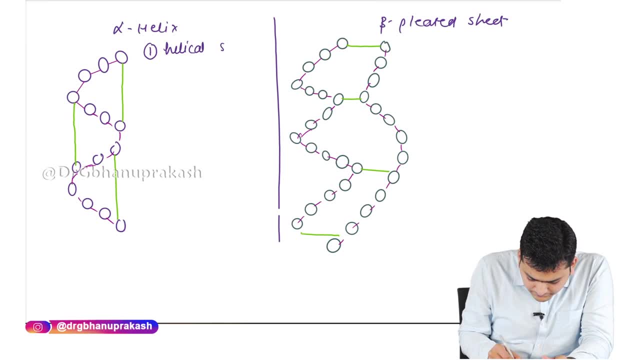 is having a helical shape, whereas the beta pleated sheet it is having the zigzag pattern. the second thing is- that is the one of the most critical point that you need to understand- in the alpha helix there is only one chain that we are having and inside the chain we are making the bond right, whereas in the beta pleated sheet there is. 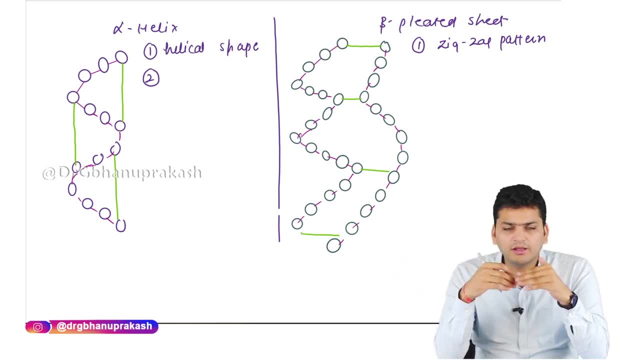 more than one chain and in that we are making the bond. so if you are making the bond inside a single chain, that is called as intra chain linkage. that is the intra chain linkage, whereas in the second one it is the inter chain linkage. in the beta pleated sheet we have the inter chain. 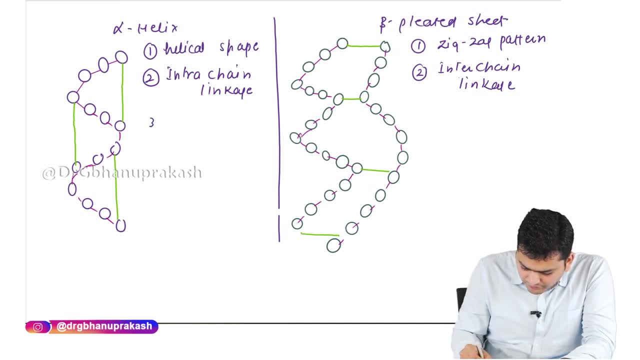 linkage. there is more than one chain and we are making the bonds. now let's see the third difference. what is the third difference is, if i ask that, which is which one seems to be more stable? right, the more stable structure is not the beta pleated sheet, it is the. 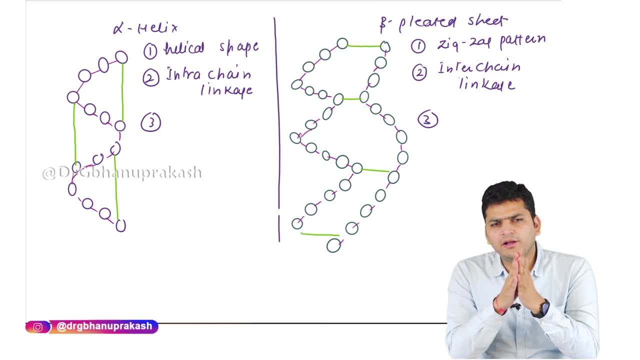 alpha helix. now why it is so? because the non-peptide relationship that is there, the non-peptide relationship is not a strong bond. the green color bond which you can see in the diagram, they are not the strong bond. they are not the strong bond. so if you just give a slight pressure, 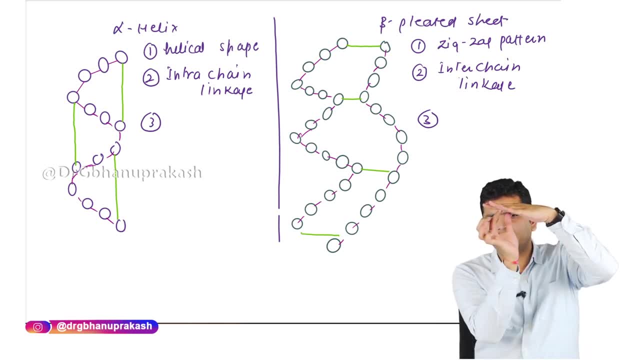 on the beta pleated sheet. see, this is the first chain. let's say this is the second chain and the bond that is there in between is the, the non-peptide relationship. so if i represent the non-peptide relationship by this plane, this is the first chain of amino acid. 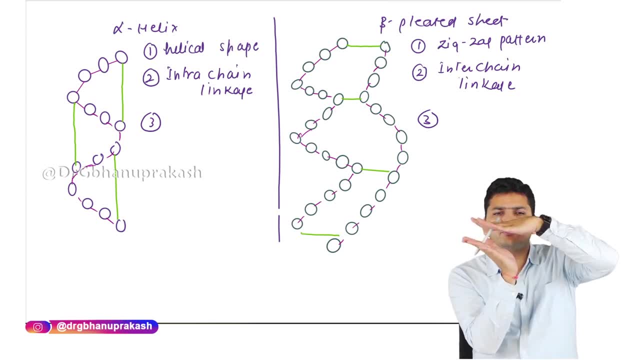 then the non-peptide and this is the second one. and this bond is not stable. if you give a slight pressure, the bond will disrupt and these chains will slip on one another, whereas in the alpha helix there is only one gene and in that you are making that bone so, despite it, will rupture or not rupture. 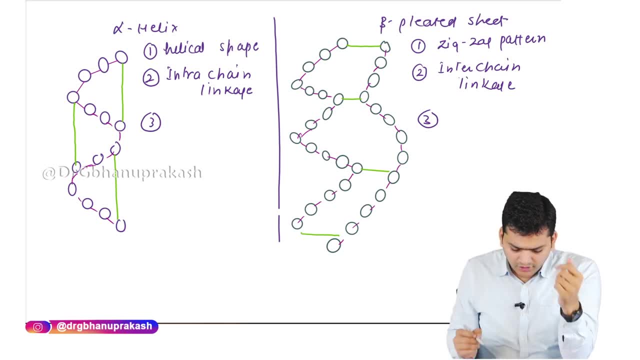 the structure will more or less will remain the same right. so i can say that alpha helix is more stable. the beta pleated sheet is less stable. if it is more stable then i can say it will be more commonly found in the body because it will live long, whereas beta pleated sheet is less common. 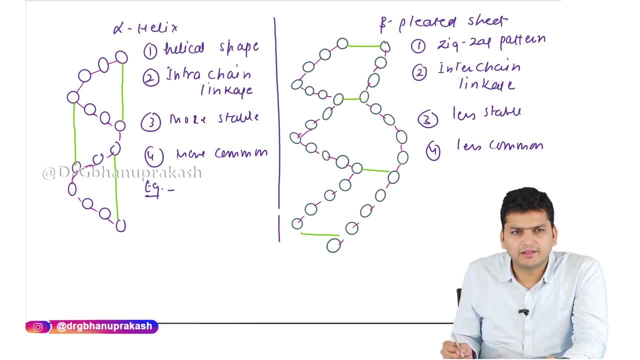 when it comes to the example of the protein which is found in alpha helix, it is the, the protein of the rbc, that is the hemoglobin, or i can say the myoglobin, the protein part, that is the globin that is found in the alpha helix form. where is the alpha helix? 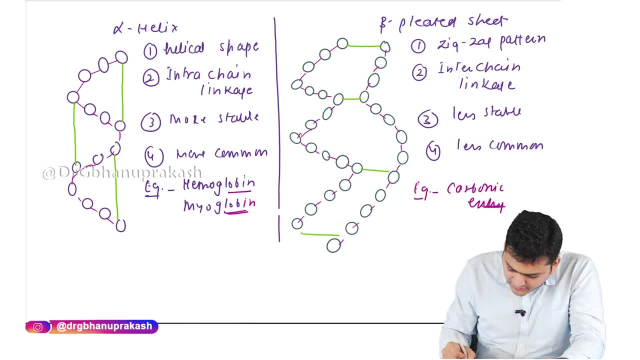 example of the beta pleated sheet is carbonic anhydrase, whereas the example of beta pleated sheet is carbonic anhydrase- carbonic anhydrase. so these are the difference between the alpha helix and the beta pleated sheet. now we'll see the, the third and the fourth subtype of the secondary. 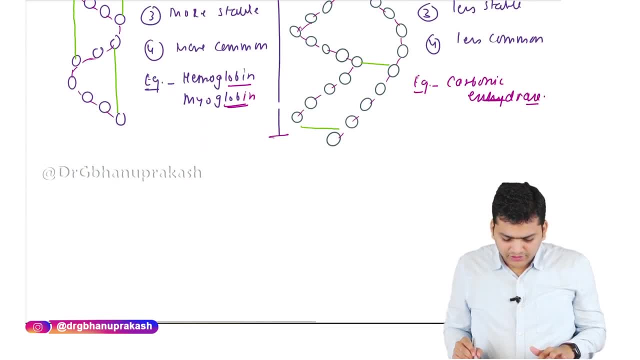 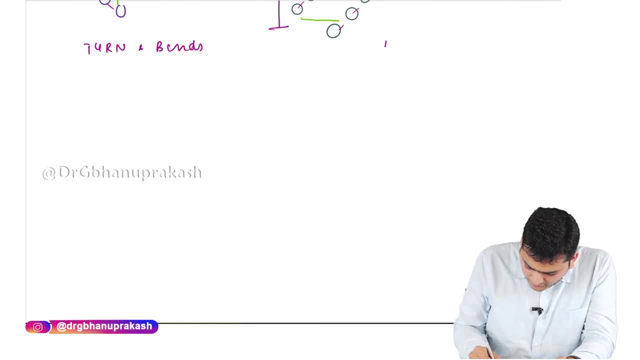 structure, that is, turn and band and the loops. so again, we'll make a differentiating table between these two: turn, band and the loop. so what are the difference between turn, band and loop, and what? what is the basic concept behind? so, to understand this, let's understand first the turn and then we'll go to the loop side. 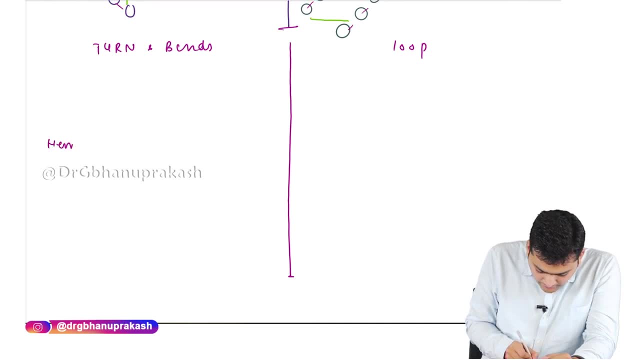 for example, just now we have discussed that- the hemoglobin, the protein part of the hemoglobin, that is the globin part. basically it is found in the alpha helix form, right. so i can say, let's say this is the one of the globin chain that we are having. 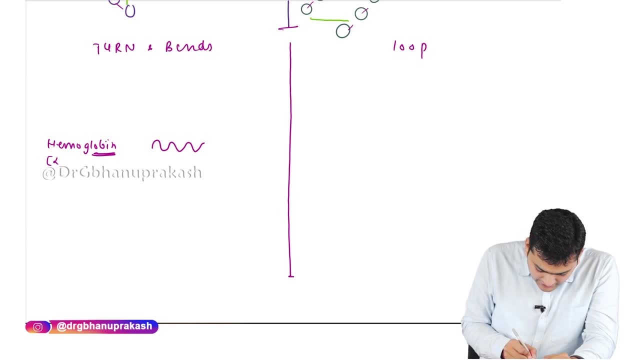 that is in the alpha helix. alpha helix means the secondary structure, alpha helix means the second structure. so i have taken a protein which is in the secondary structure, alpha helix. taking one more hemoglobin molecule again, this globin part is going to have the alpha helix form and that is. 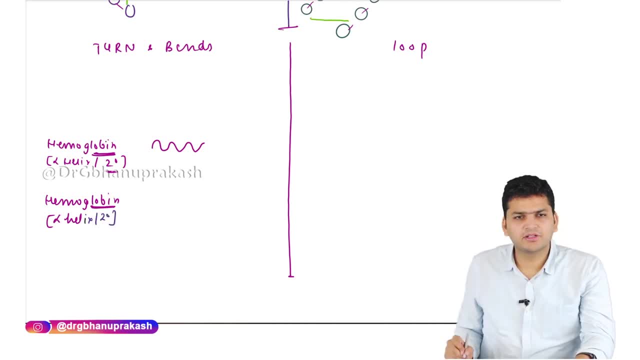 going to be the secondary structure. that is going to be the secondary structure. so that is again. let's say, this is one more protein that is in the secondary structure. now i want to join these two secondary structure. what i want to do is i want to join these two secondary structure. if i want to, 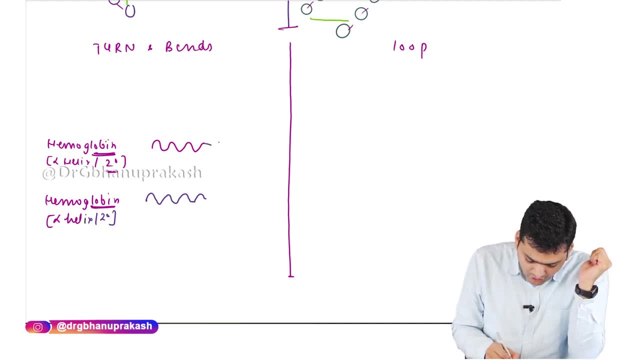 join these two secondary structure. what i can do is i can take a short chain of amino acid. a short chain means three, four amino acids are there and via this short chain i can link these two secondary structure. if i join two secondary structure via a short chain of amino acid. 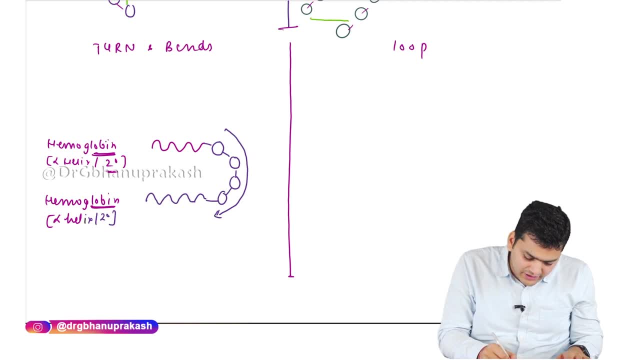 via a short chain of amino acid. this short chain of amino acid is referred as turn and band is referred as turn and band. so what is turn and band is a short chain of amino acid which joins to secondary structures. a joint two secondary structure is called as the turn and back. when it comes to 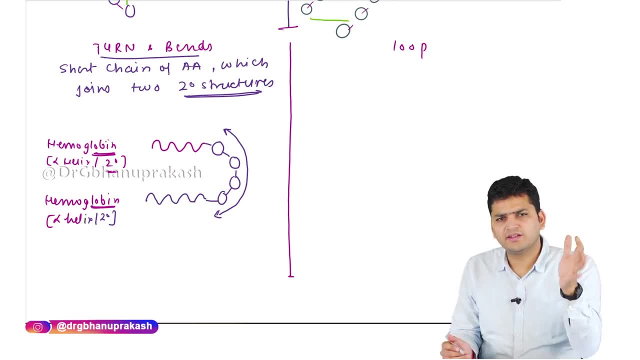 the. when it comes to turn and bend, we understood. the concept is very easy: that we want to join two secondary structures and we are using a short chain that will be referred as turn and back. now the question they ask is which amino acid are commonly found in turn and band, or which amino acid are going to make the turn and back The. answer is going to be proline and glycine. so let's write down this point is: turn and band are commonly made up of proline and glycine. turn and band are commonly made up of the amino acid that is going to be. there is proline and glycine. these are the amino acid. 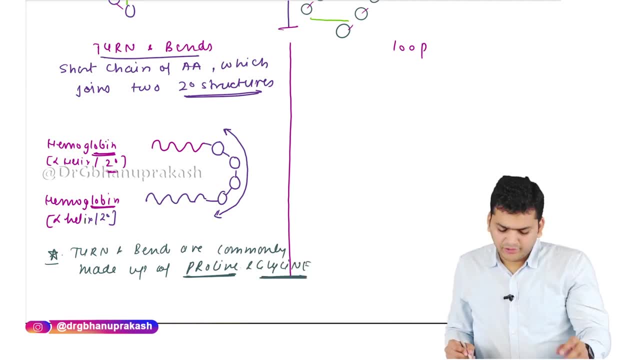 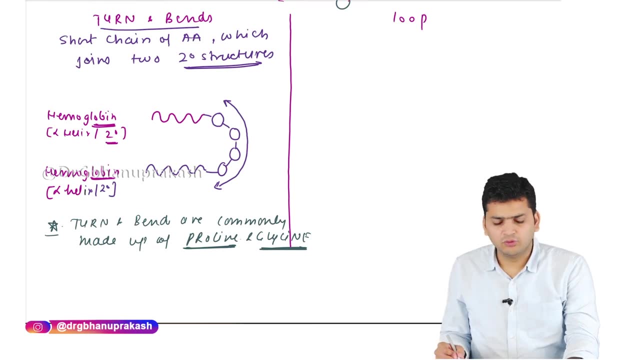 that we are going to see in the, in the turn and band. now, when it comes to the loop, when it comes to the loop, let's say, to make you understand the loop, what i am saying is, again, i am taking the same example. same example means i am taking the hemoglobin molecule. 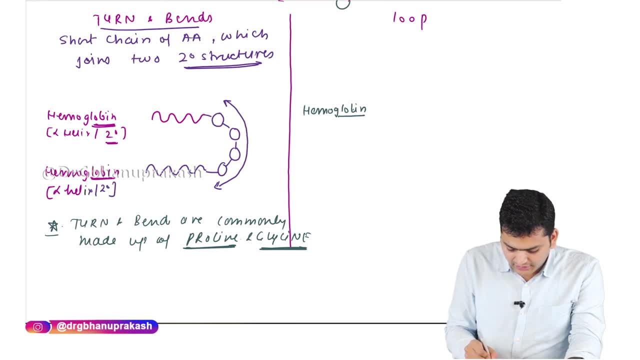 we know that the protein part of hemoglobin is found in the secondary structure, alpha helix form. so let's say this is the alpha helix. i am taking one more hemoglobin molecule, the secondary structure, the alpha helix form. let's say this one. now i want to join it. so 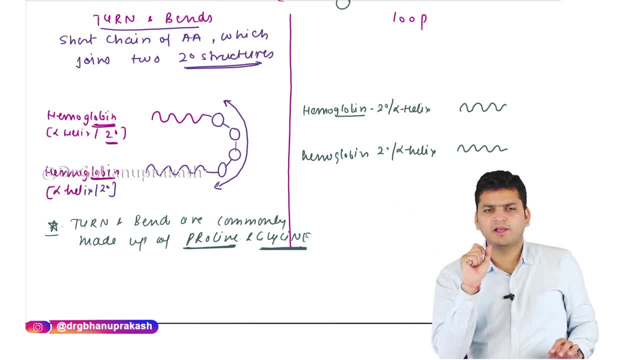 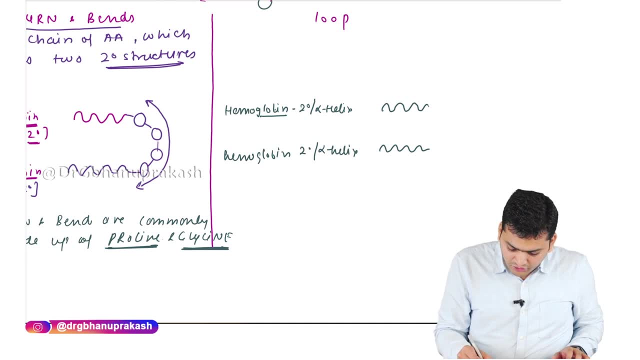 i will join it in turn and band. what i did is i have taken a short chain by which we have joined these two secondary structure. this time, when i want to join these two secondary structure, what i do is, instead of taking a short chain, i take a long chain of amino acid. 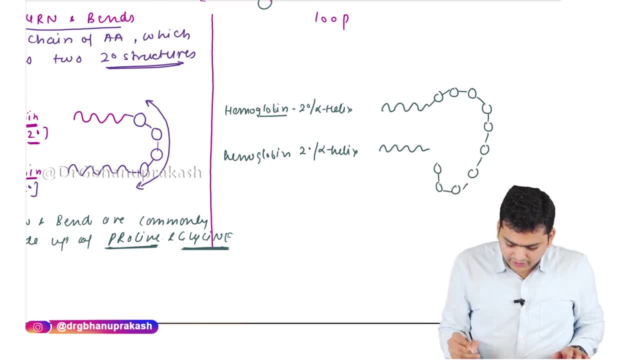 if i take a long chain of amino acid by which we are joining these two secondary structure, this long chain is referred as loop. so turn and band and loop are very similar. it is only the size which is different. turn and band, it is a short chain and loop is going to be. 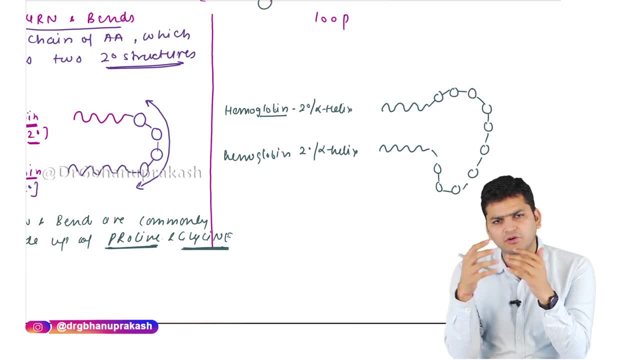 a large chain. so i can say alpha Shit daisini from alpha helix form and hom nouvelle proline from helix pattern from space haög embic licensing form from space ha, épisode part, ugh hk. I can say L for the larger version of turn and bend. so let's write down this point that. 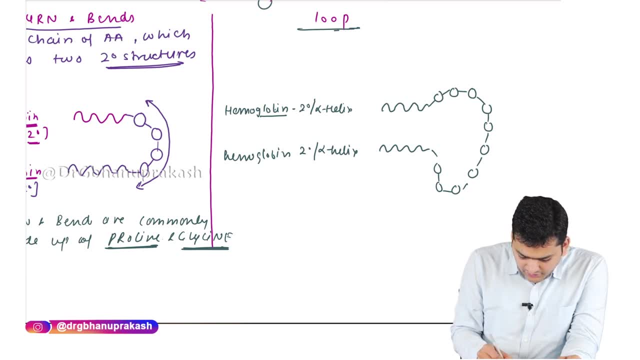 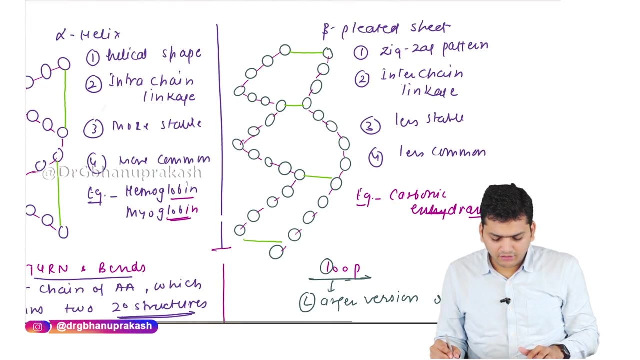 what is loop is is the larger version of turn and bend, larger version of turn and bend that is referred as loop. so we have discussed all the four types of secondary structure. if I just briefly revise, the first that we have discussed was the alpha helix and the beta. 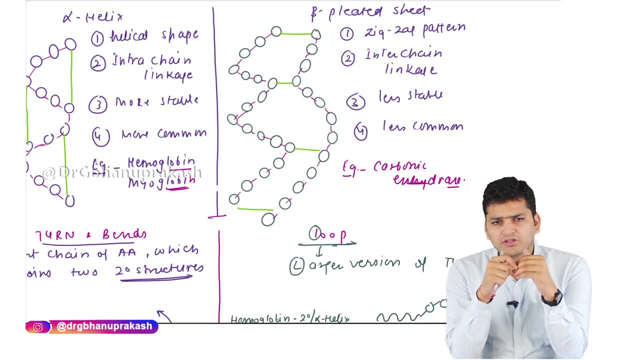 plated sheet, the most common structure. second structure that you are going to find in the body is the alpha helix. right, because the stable structure that is more common, that is more common, that is more stable. and the examples are: the globin part of the hemoglobin. 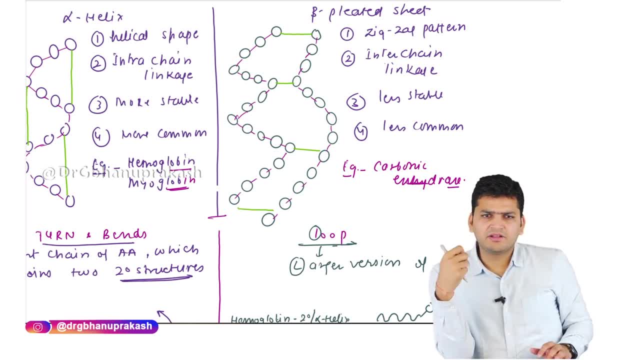 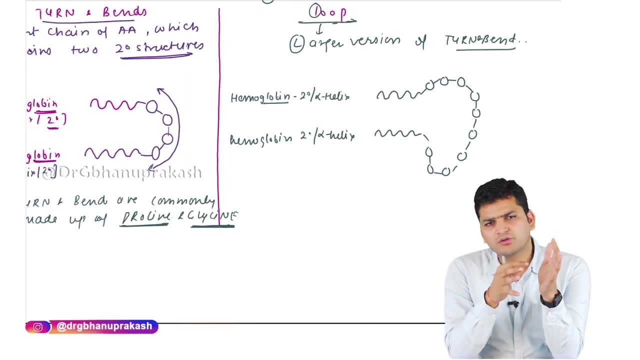 and the myoglobin, the beta plated sheet. that is less stable. there is interchange linkage and the example is the carbonic anhydrase. when it comes to turn and bend and loop, they are basically the joining units. if it is small, it is turn and bend, if it is long, it is called. 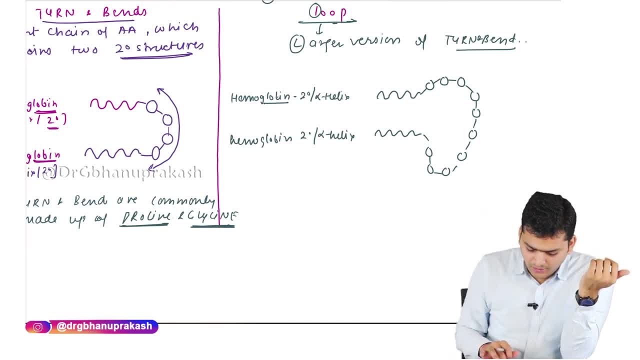 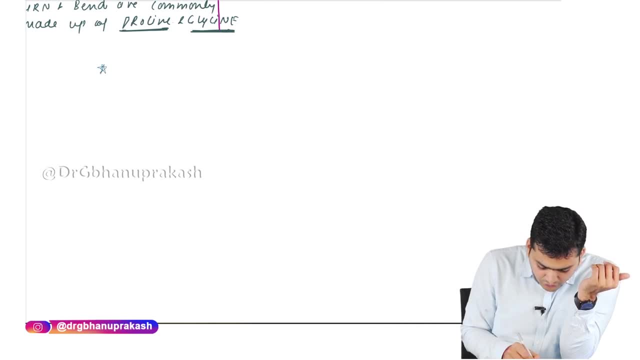 loop right. so these are the secondary structures. we have discussed all the four types of the beta plated sheet. the beta plated sheet is the one that we have now. before going to tertiary structure, I want to add one more definition here. before going to tertiary structure, I want to add one more definition here. and the 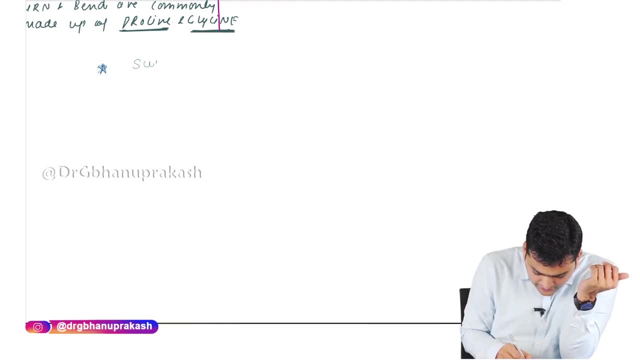 definition is of super secondary structure, something called as super secondary structure, super secondary structure. let's understand what a super secondary structure is. so, to understand the super secondary structure, what I can say is: if you have, let's say, a protein which is in the alpha helix form, if I make a protein which is in the alpha helix form, 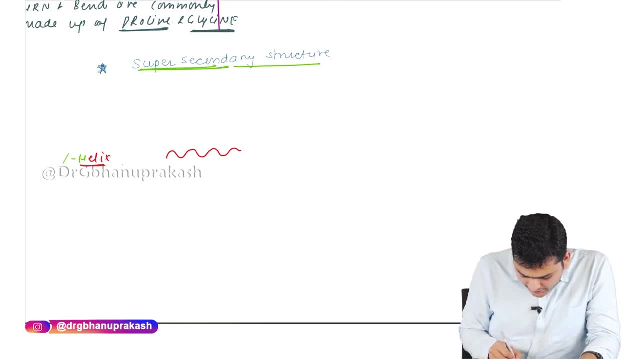 there is one more protein which is also in the alpha helix form. so basically, I have taken two secondary structures of the protein and I want to join these two secondary structures so either I can use turn and bend or I can use the loop. so, for example, if I use, for example, 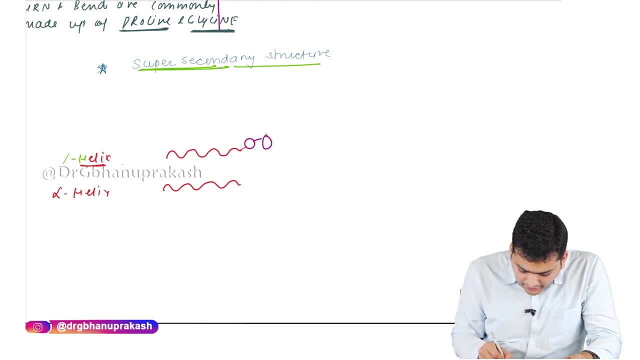 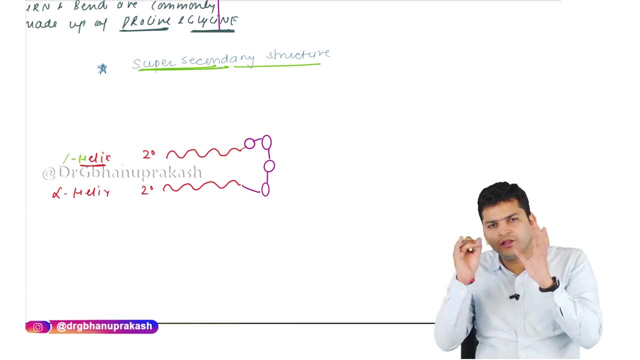 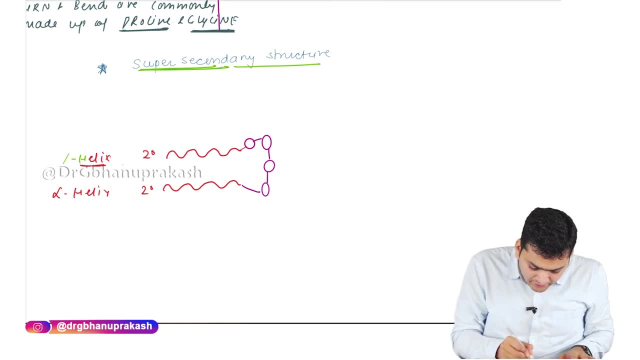 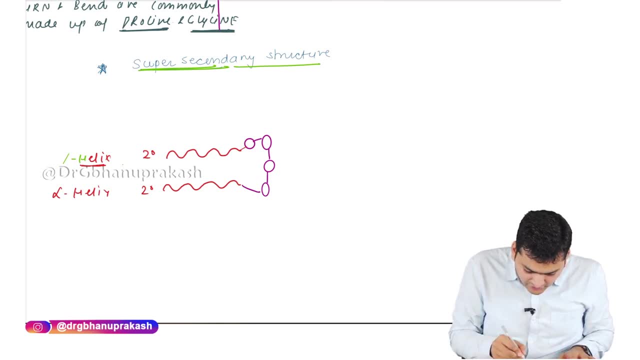 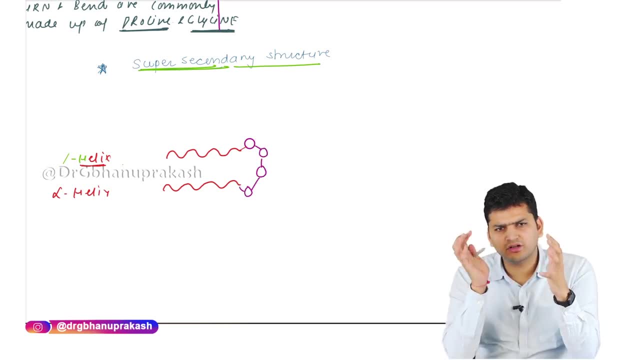 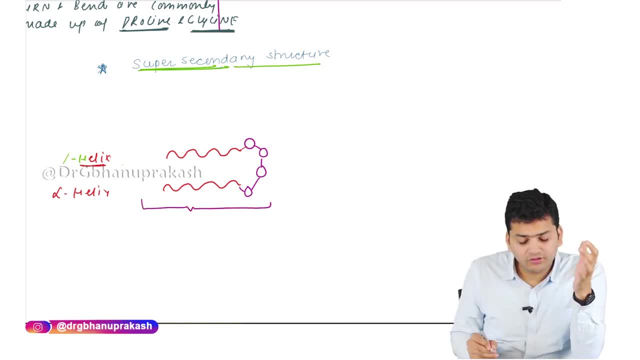 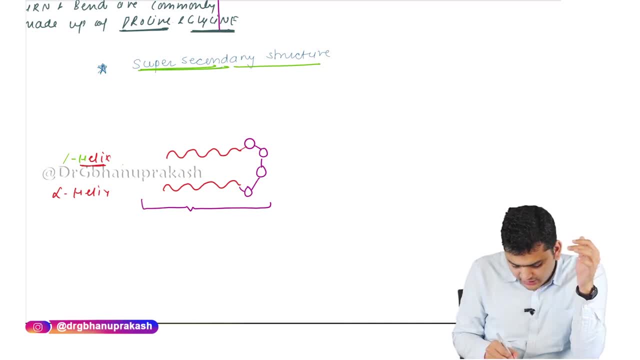 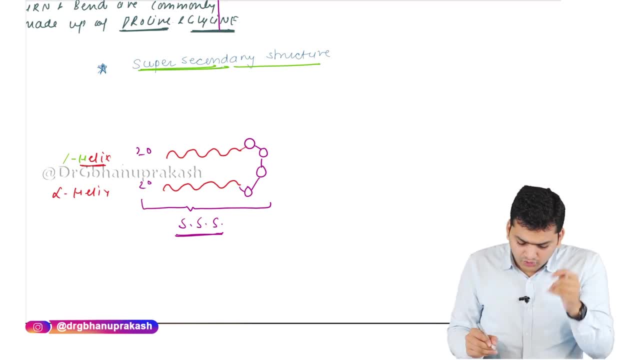 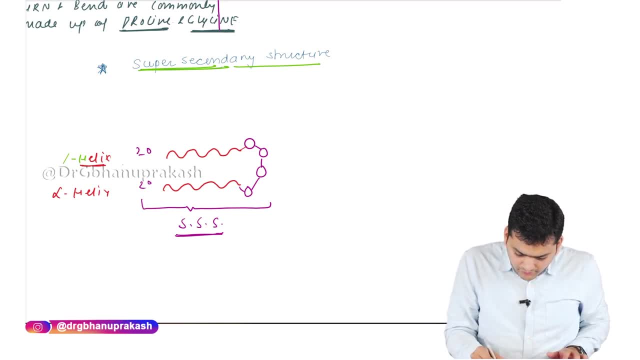 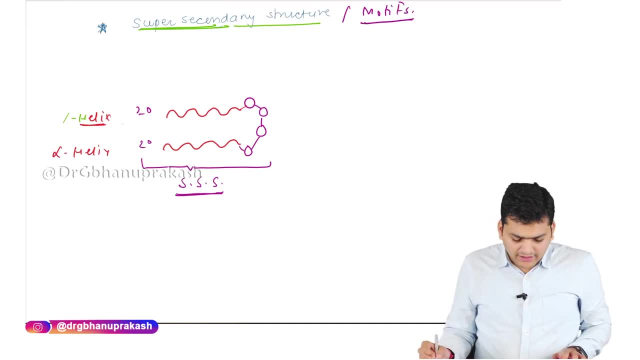 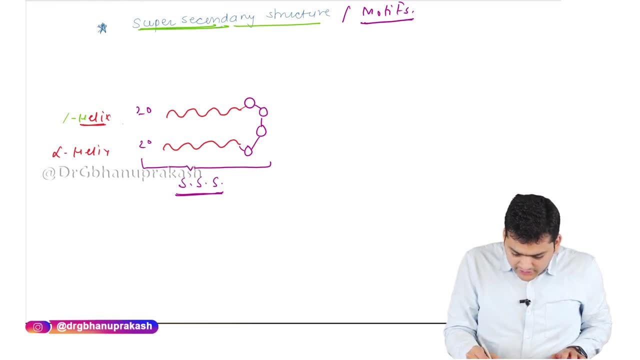 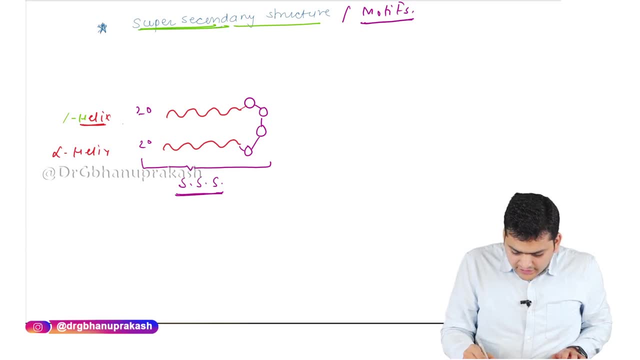 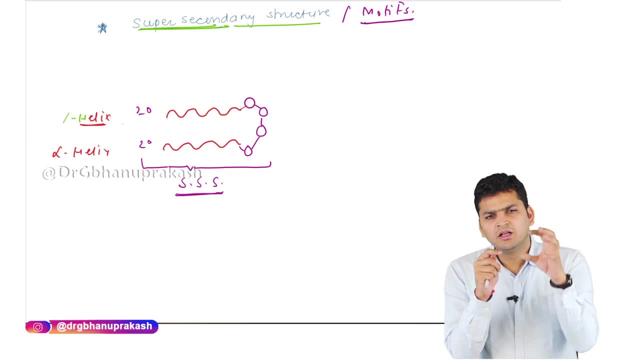 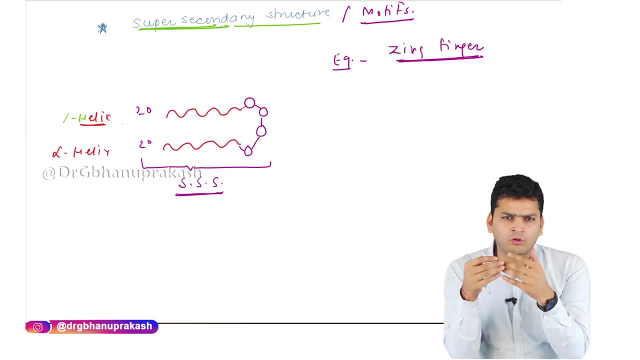 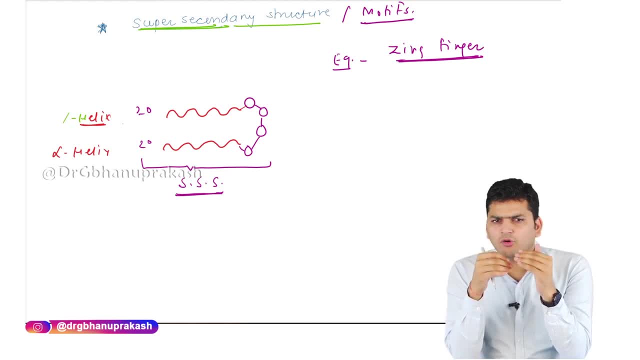 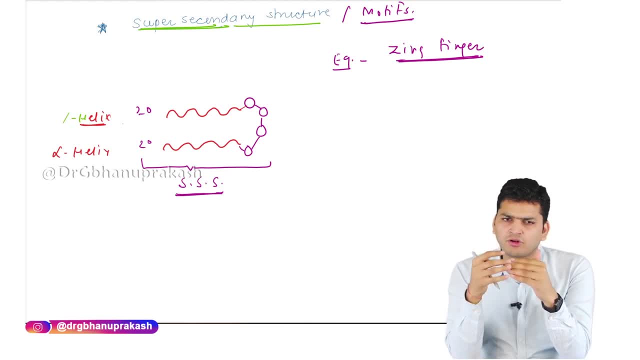 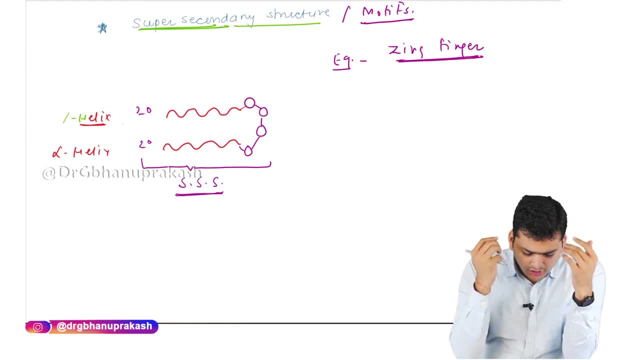 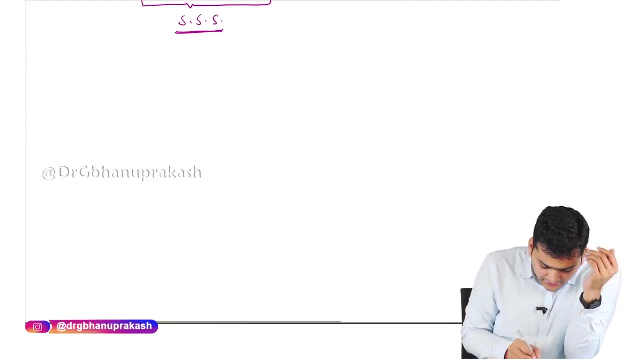 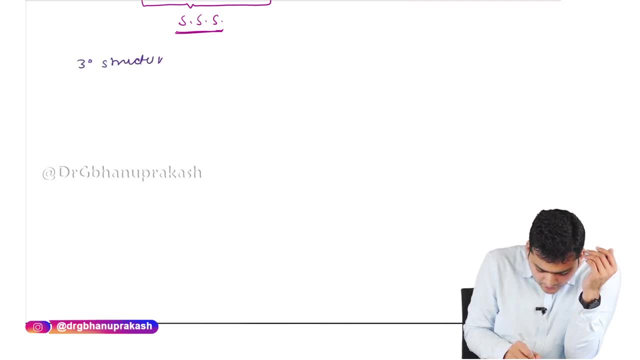 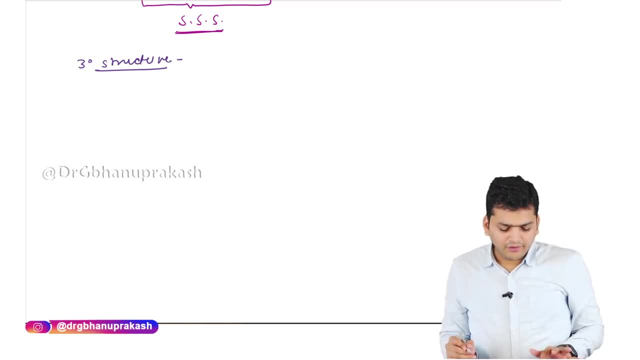 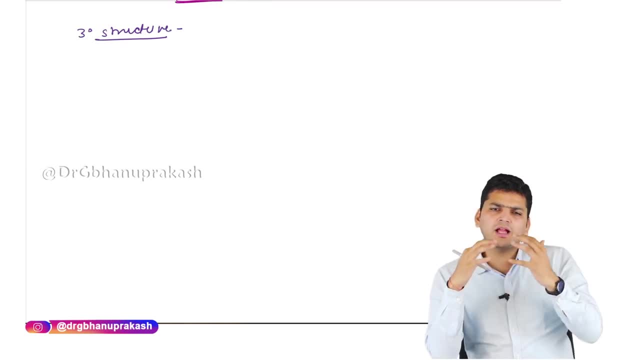 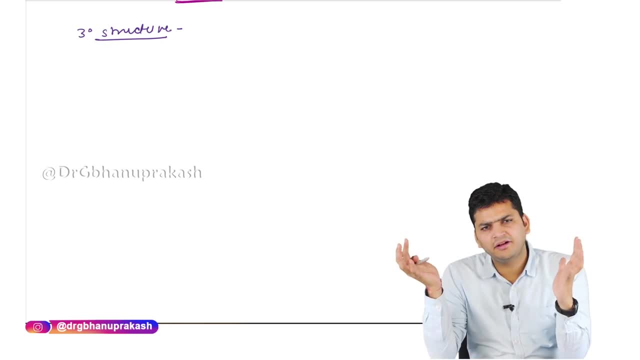 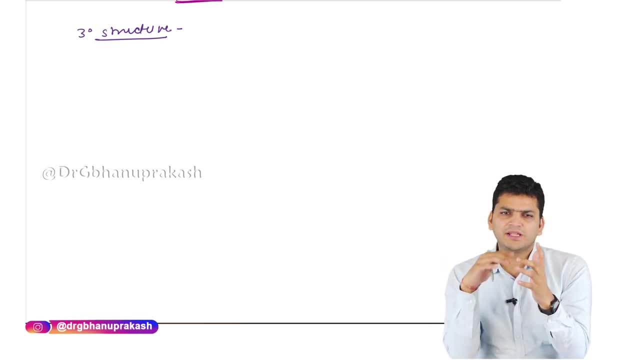 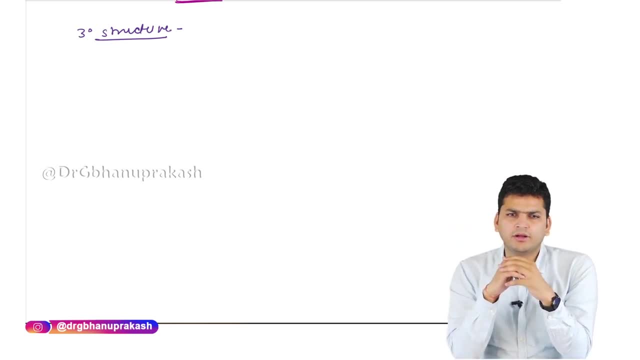 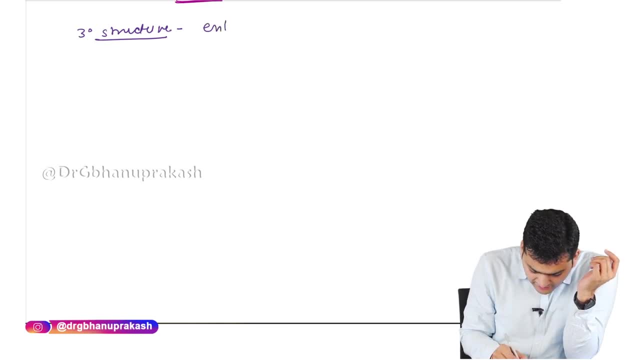 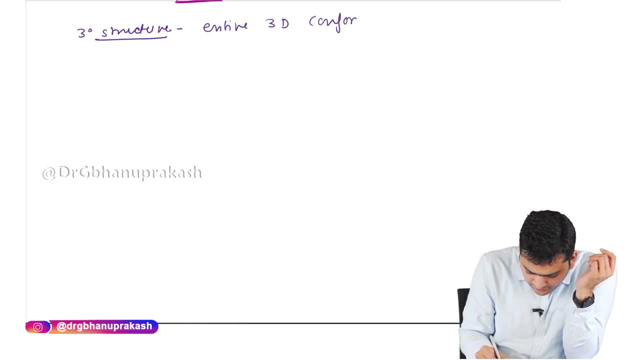 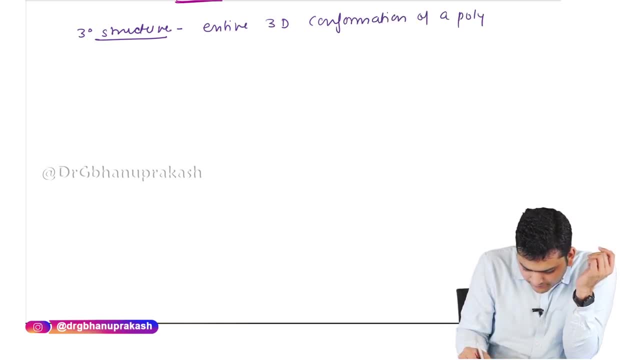 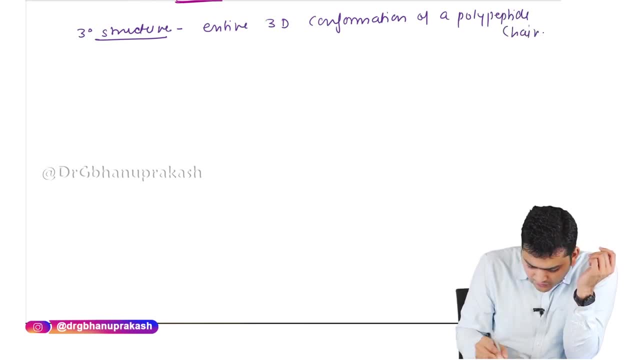 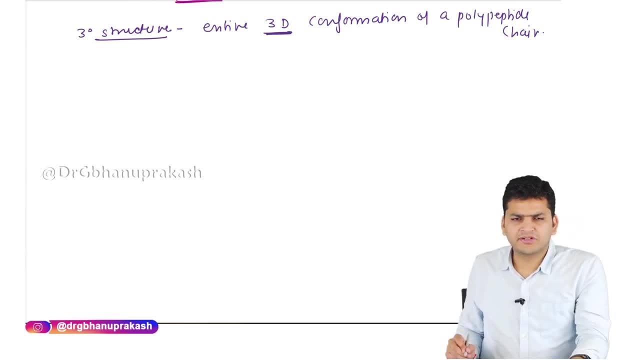 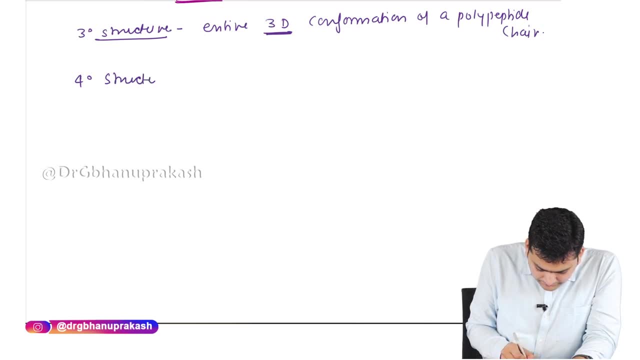 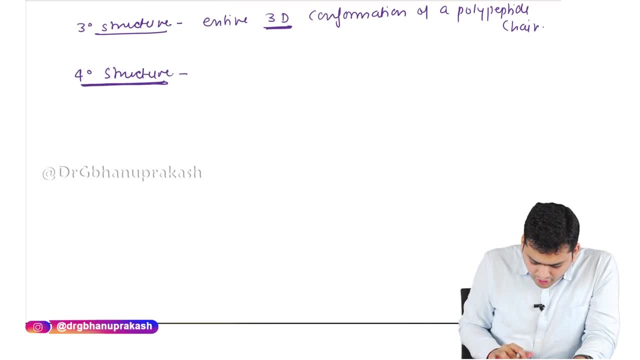 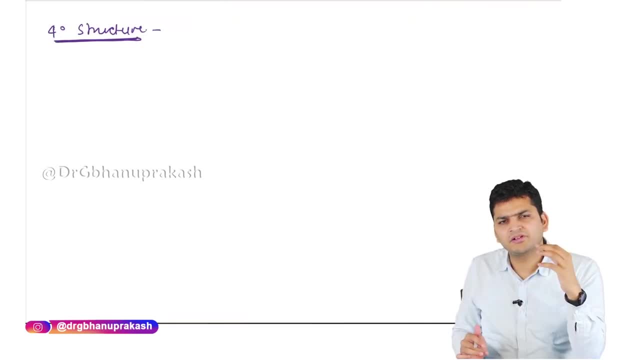 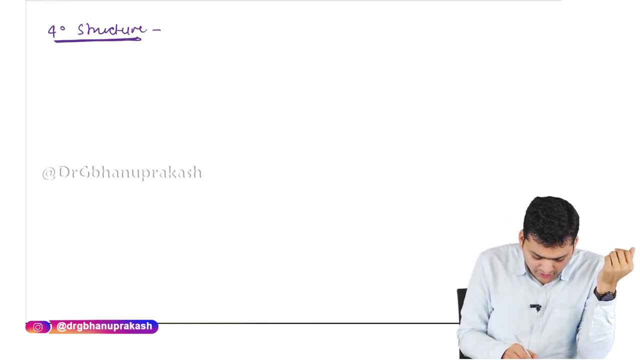 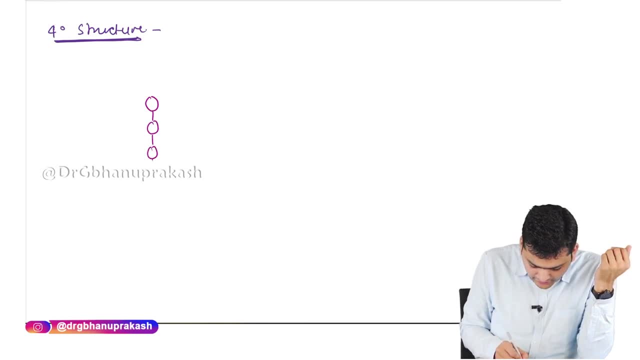 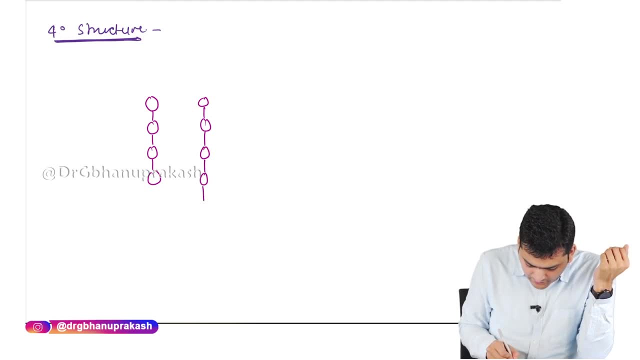 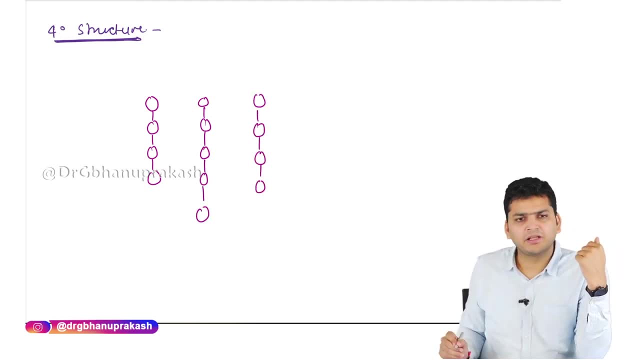 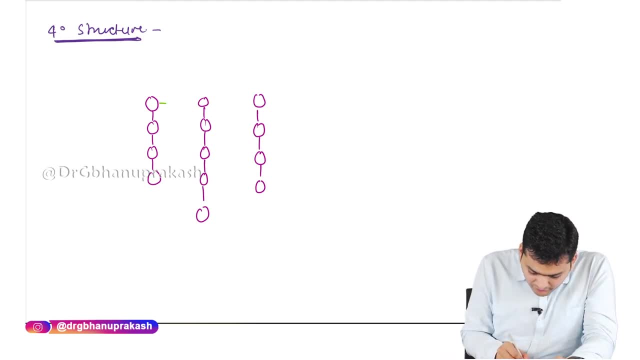 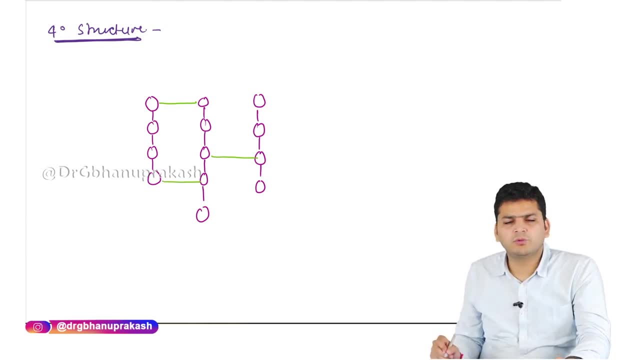 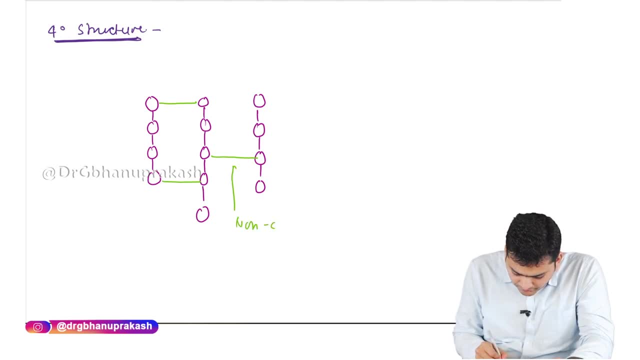 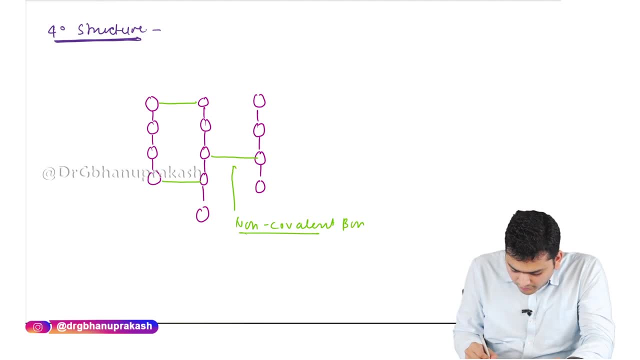 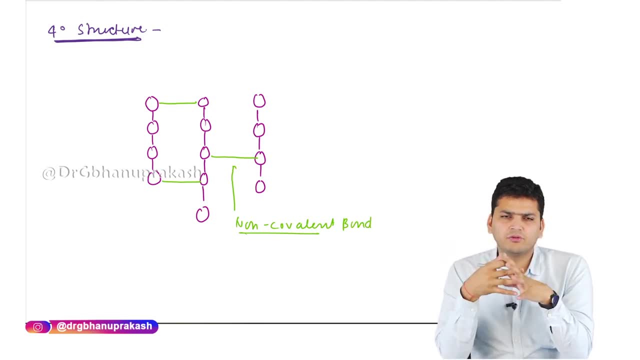 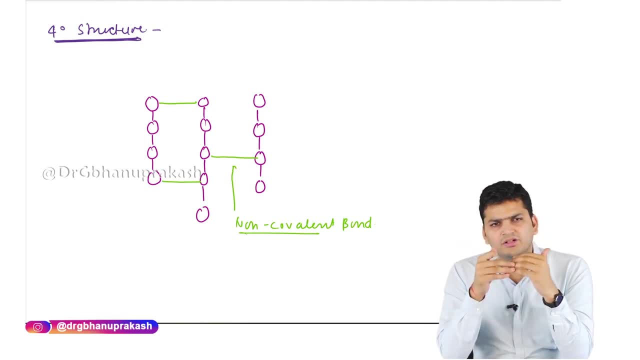 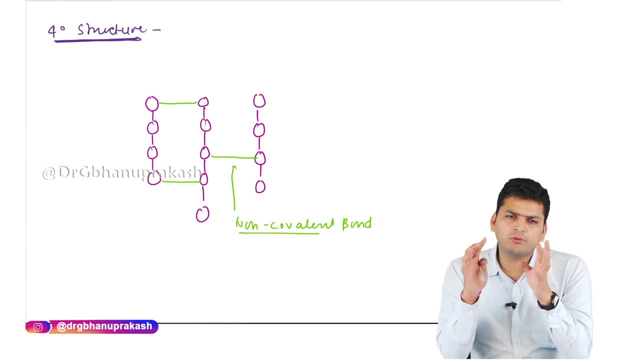 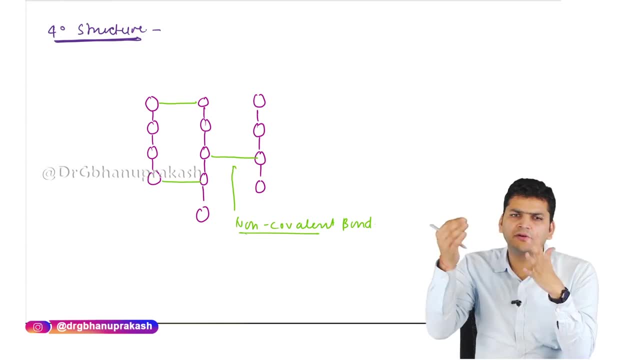 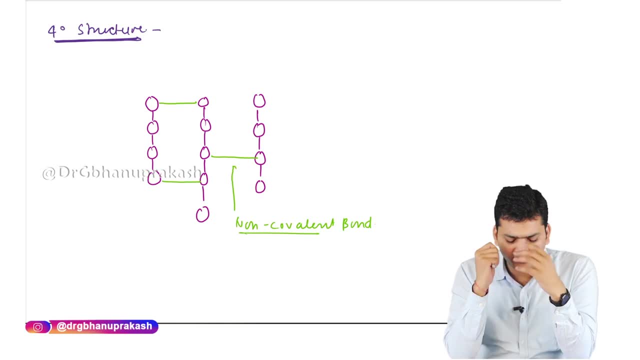 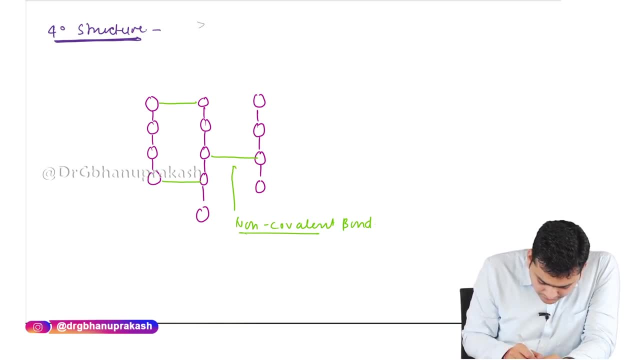 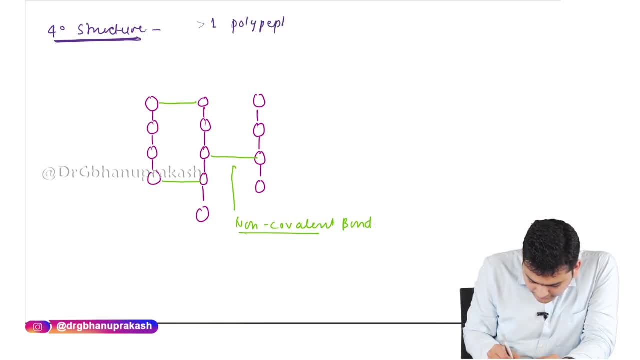 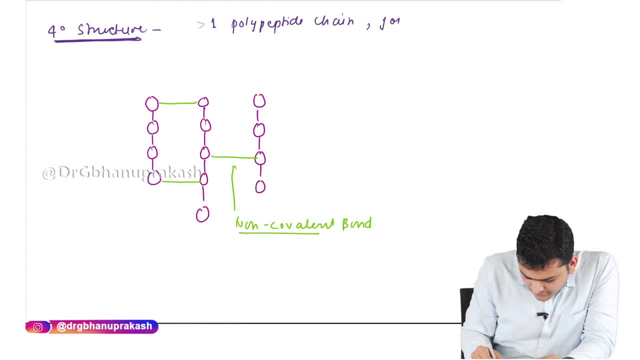 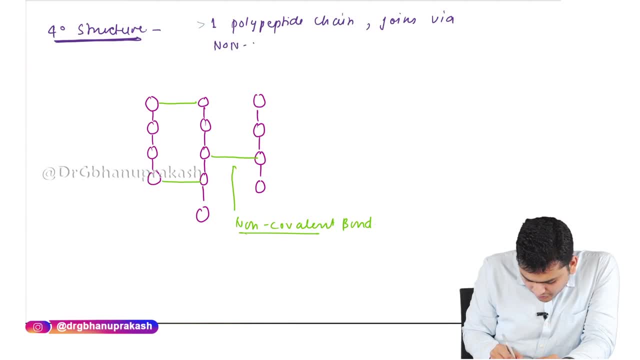 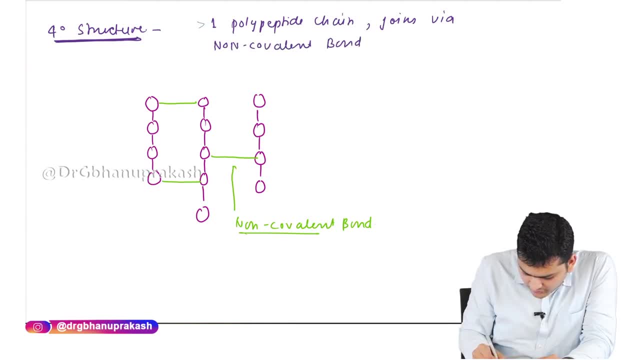 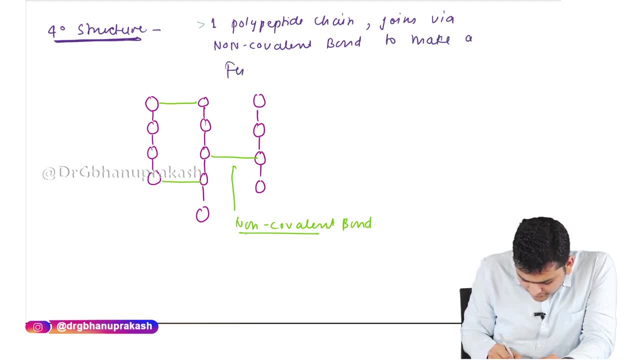 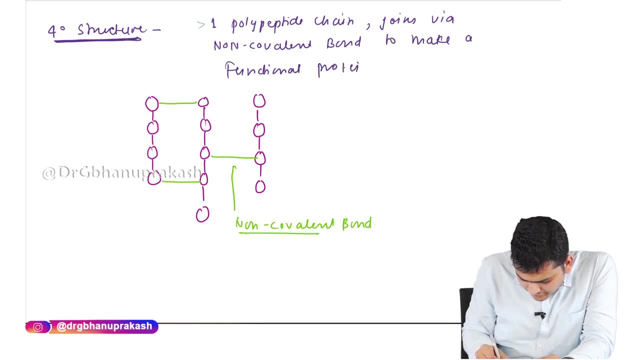 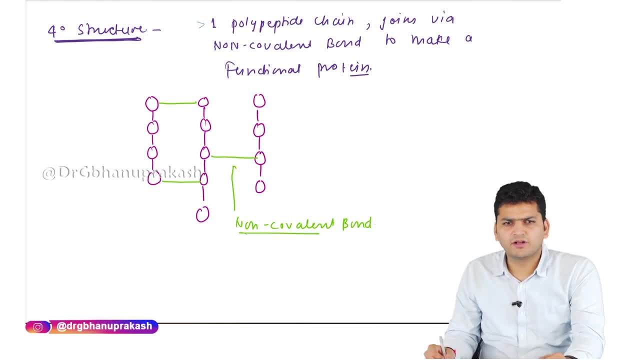 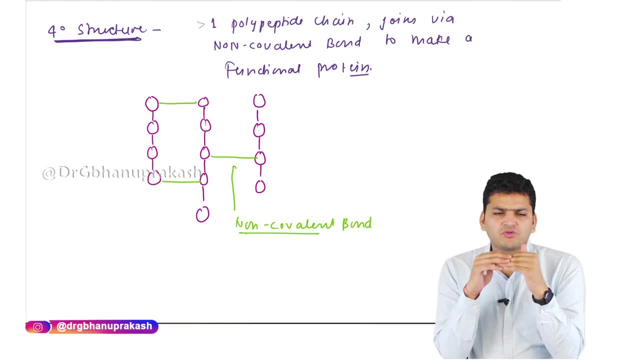 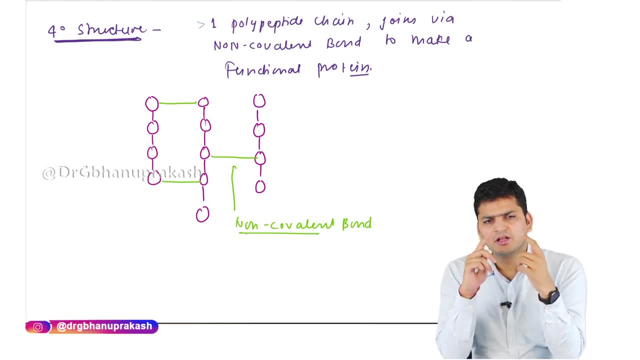 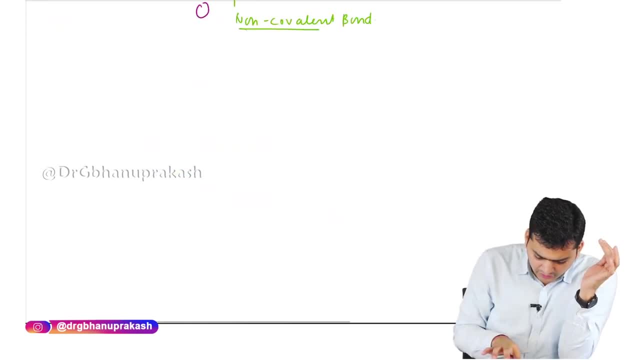 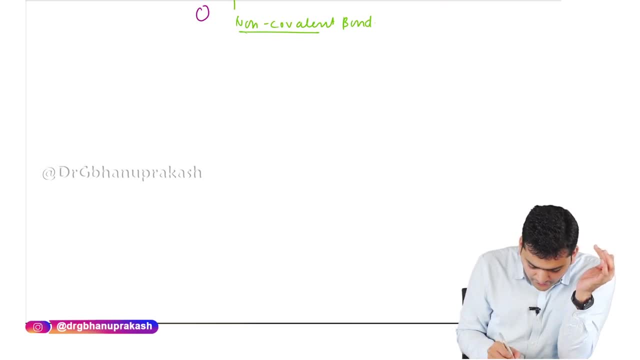 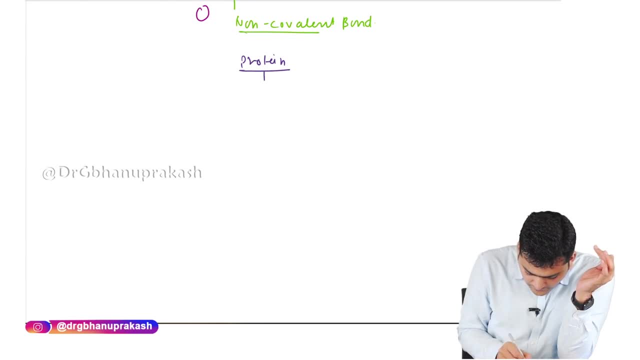 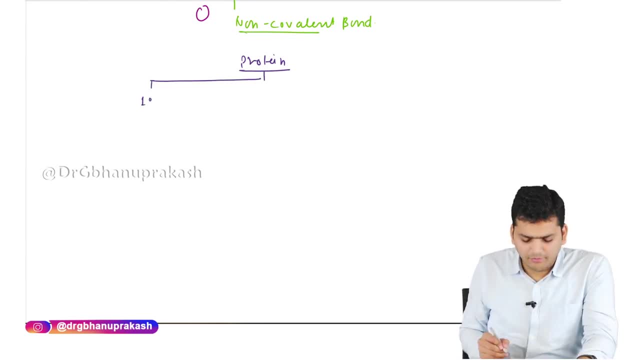 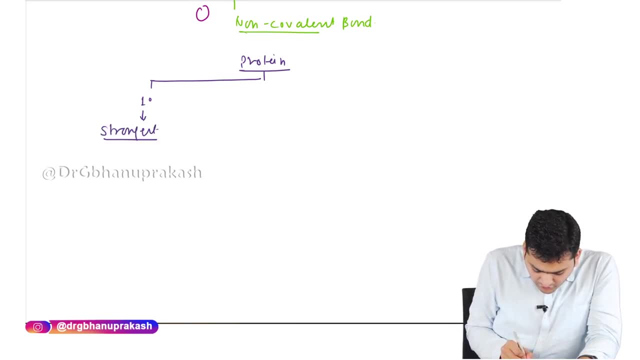 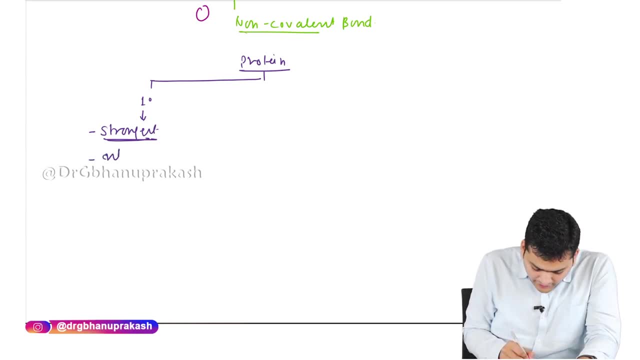 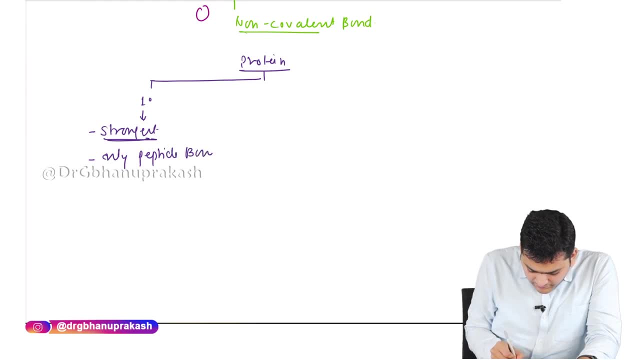 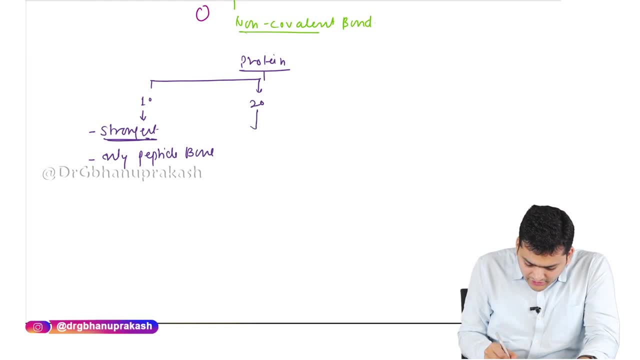 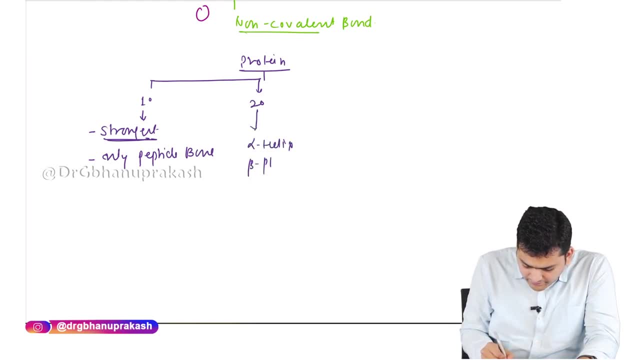 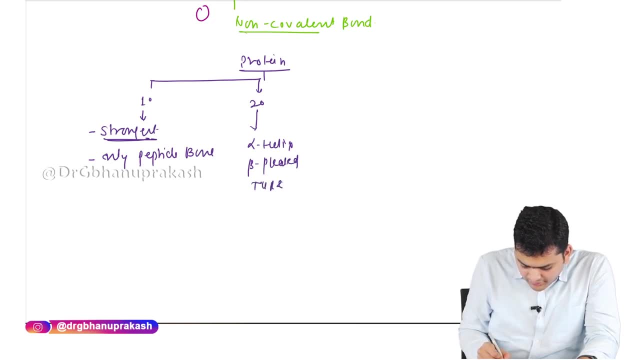 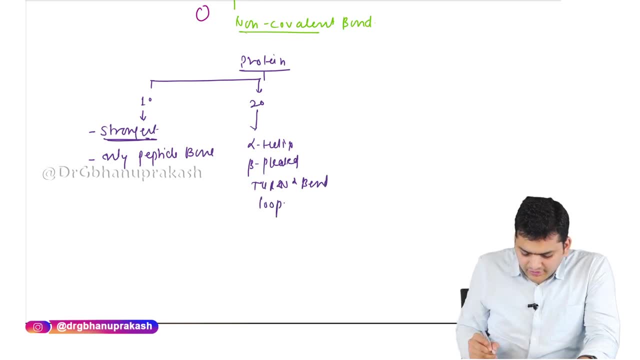 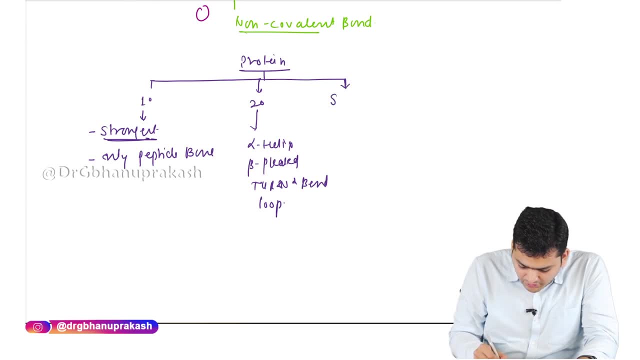 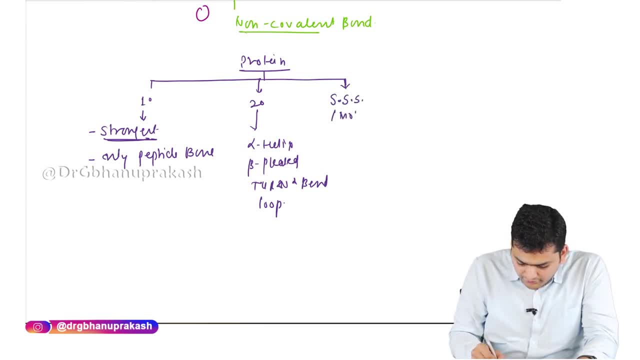 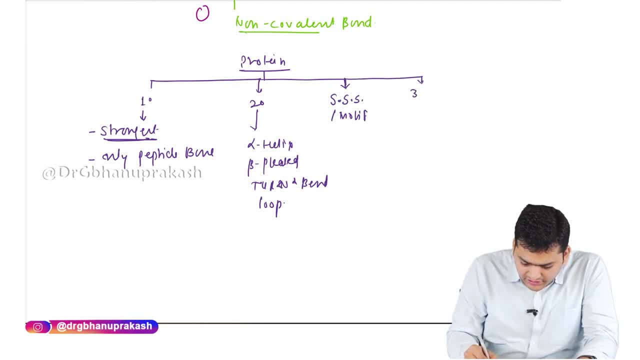 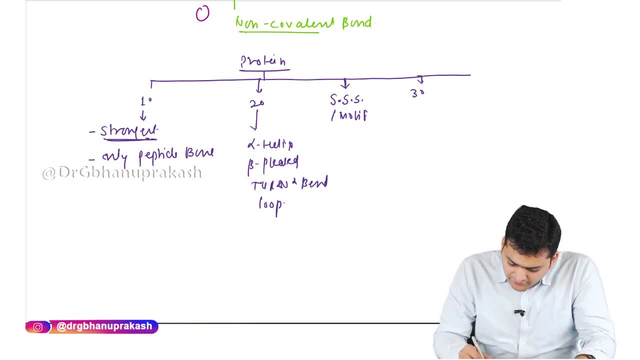 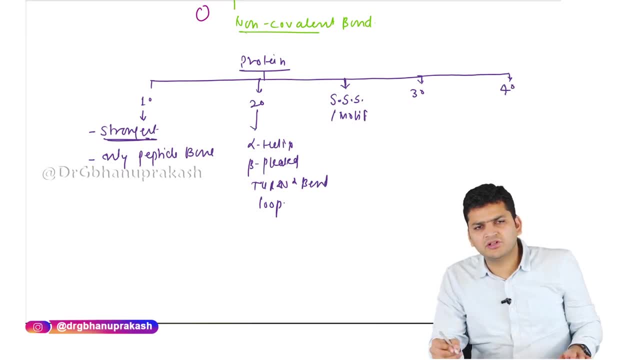 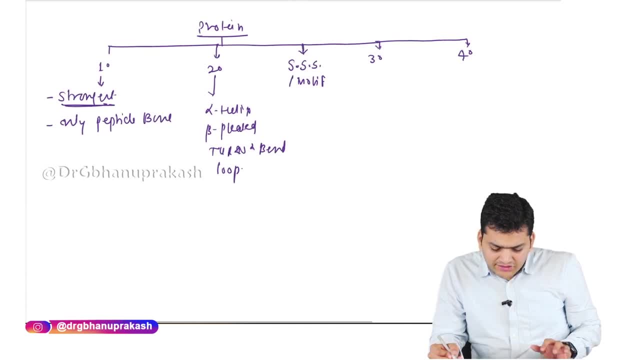 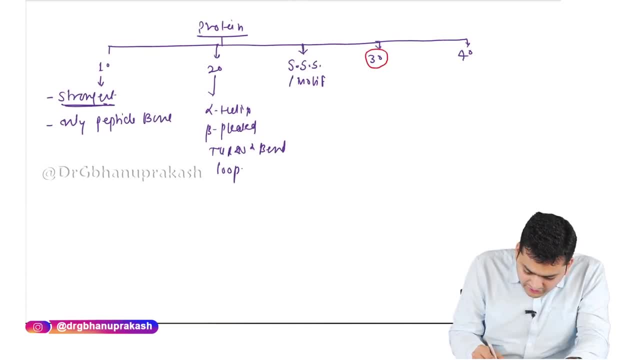 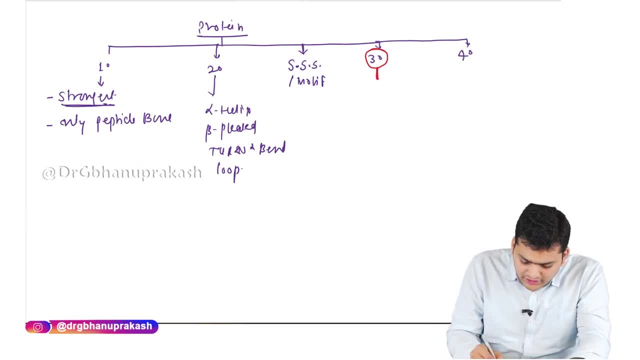 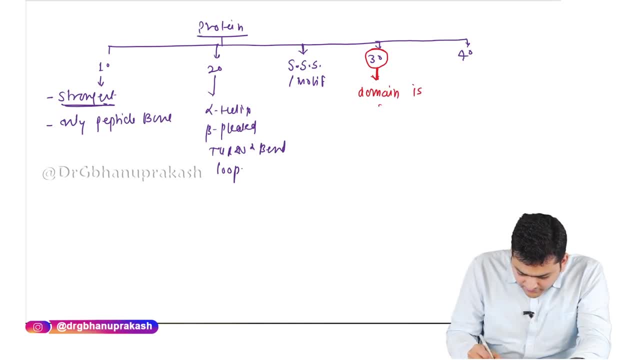 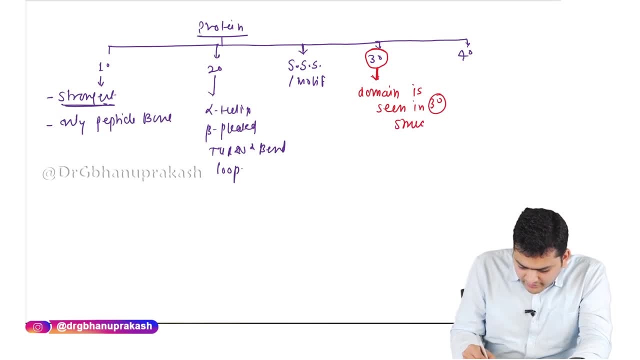 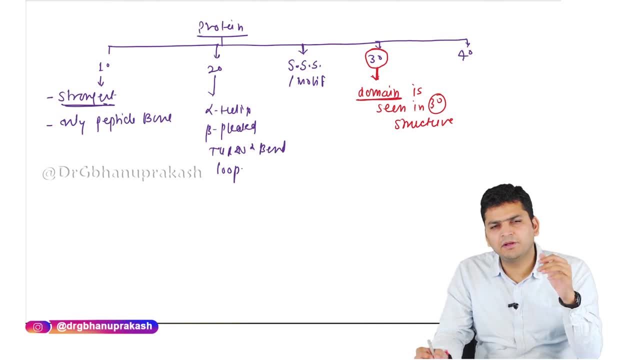 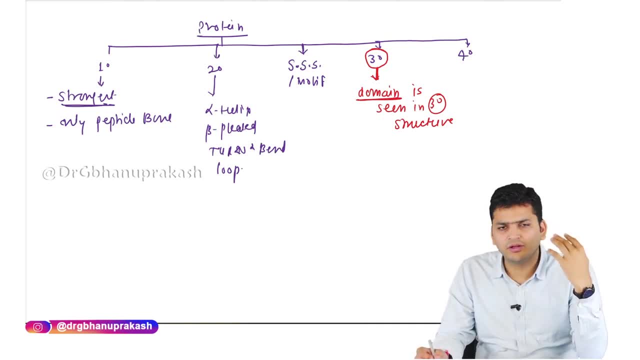 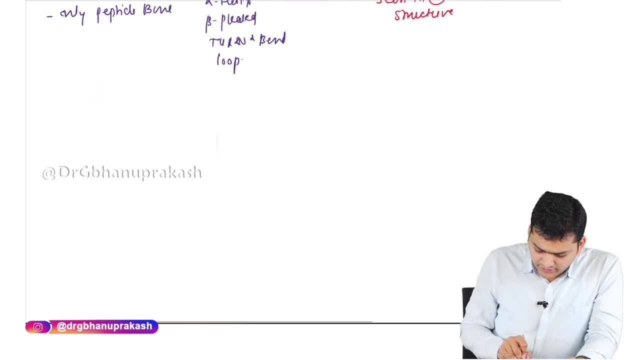 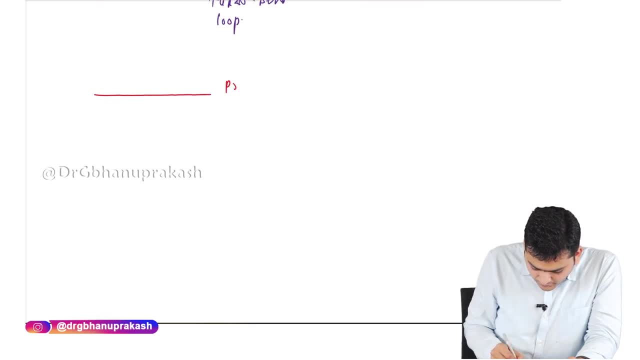 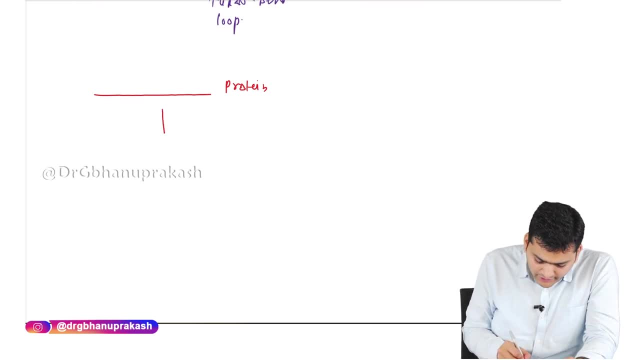 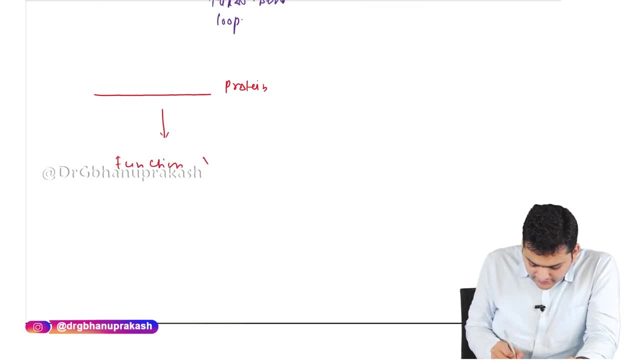 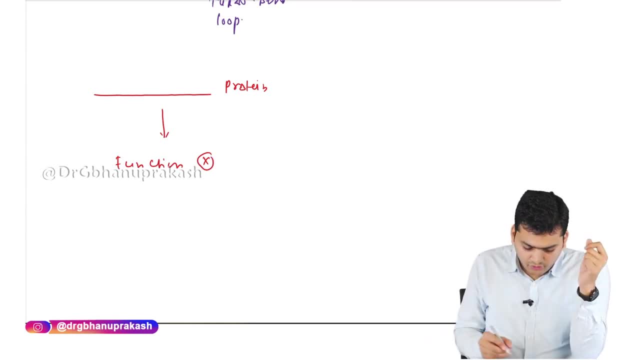 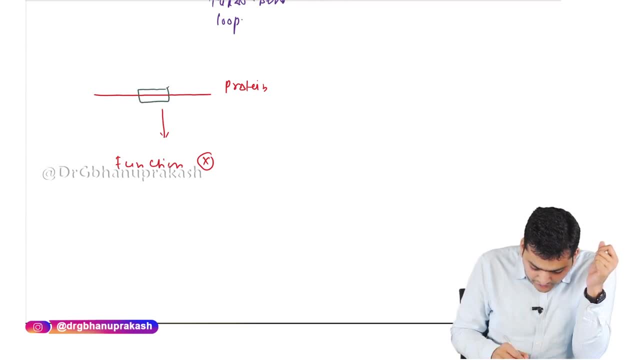 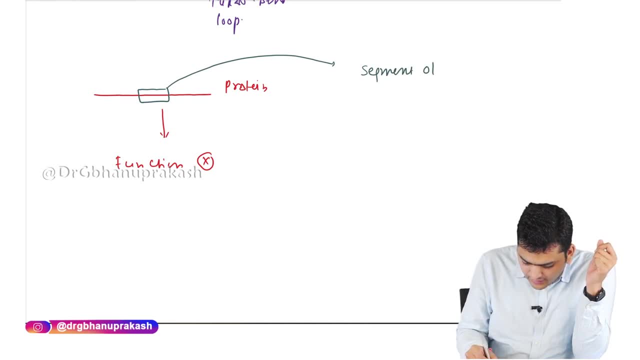 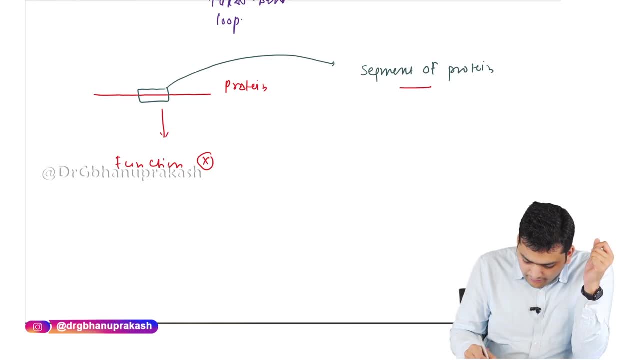 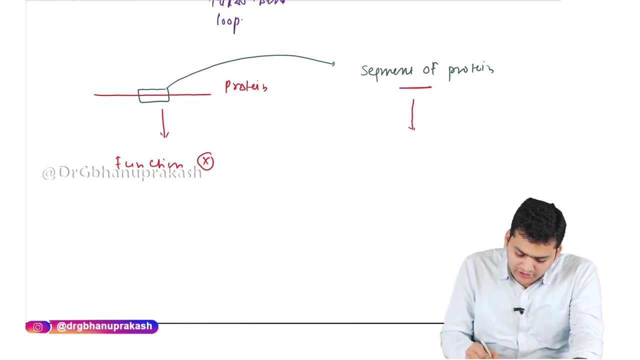 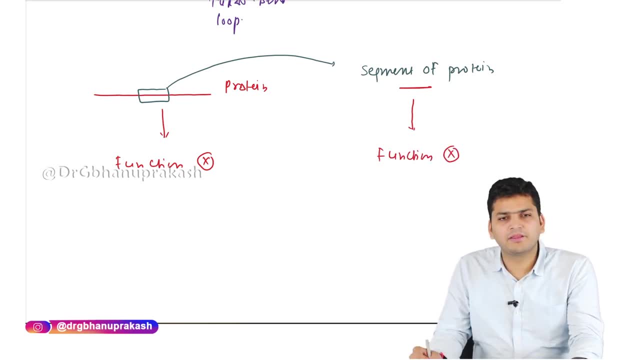 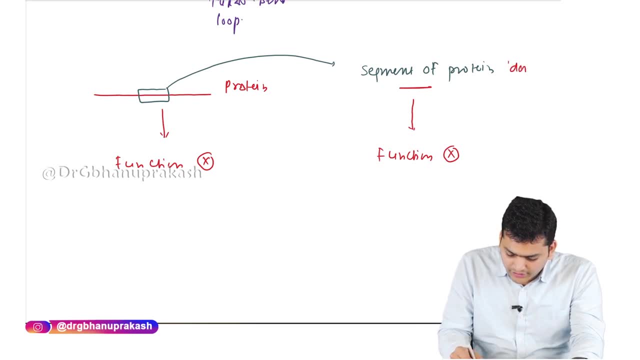 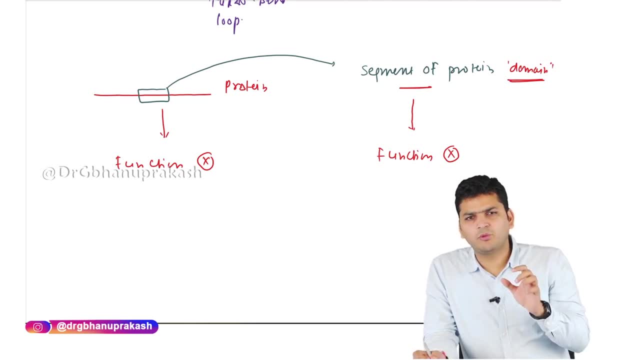 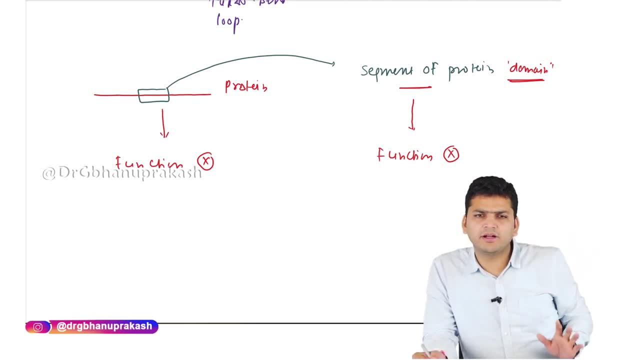 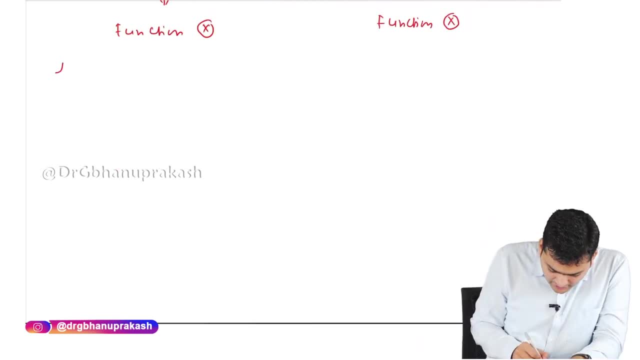 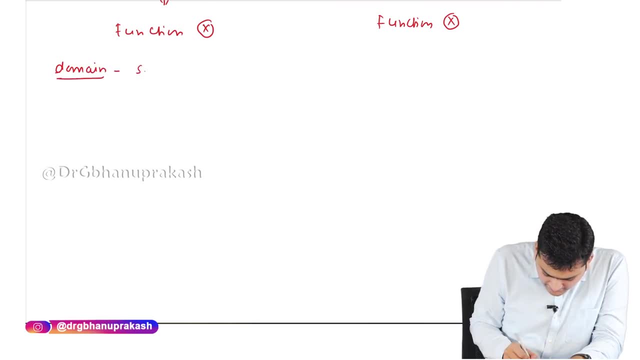 so basically, I am using a super secondary structure which is in the super secondary structure. so basically, I am using a super secondary structure which is in the super secondary structure. Domain is segment of protein which is able to perform same chemical and physical task as protein Means. whatever task that protein is able to do, that the same task this domain can also. 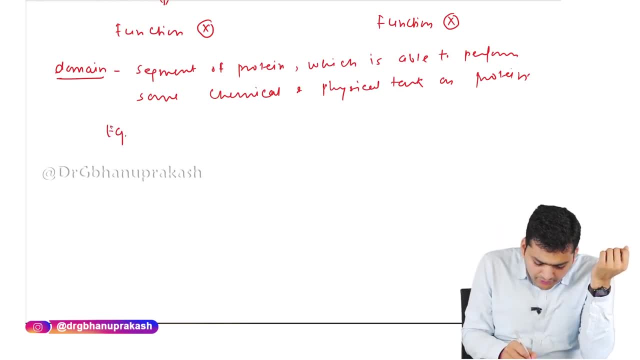 do. that is called as domain. What is the thing that you need to remember? the example of domain is something called as Rosman Fold. Rosman Fold is an example of domain where this Rosman Fold is found. this Rosman Fold is found in the enzymes of Oxido reductase category. 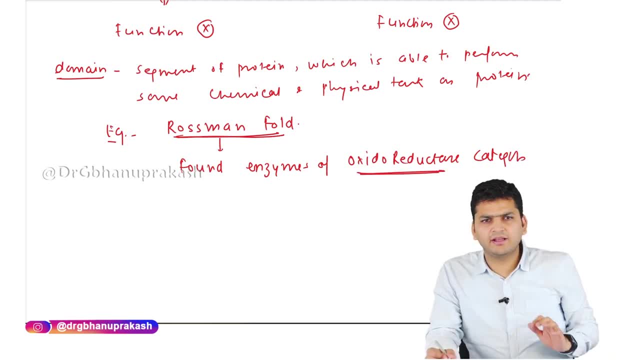 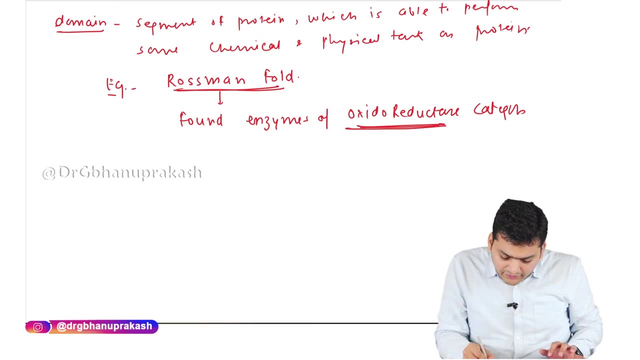 What is Oxido reductase category? See, the enzymes are divided into two categories. They are divided into 6 categories that we have discussed in the separate video where we have discussed about the different types of protein, different types of enzyme, in that the first category that we have discussed is the Oxido reductase category of the enzymes. 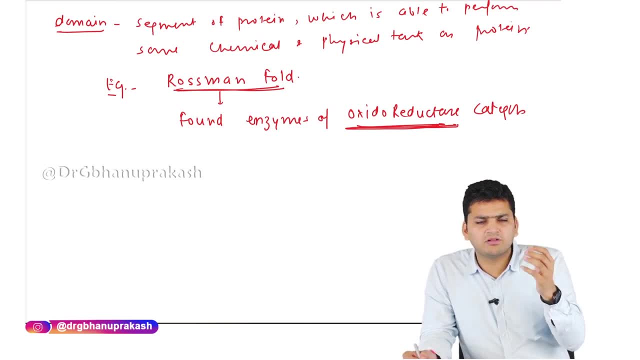 In those Oxido reductase categories of the enzymes. we have the Rosman Fold, which is the example of domain, So I just want to write one example here of Oxido reductase category enzyme, that is, Lactate dehydrogenase. 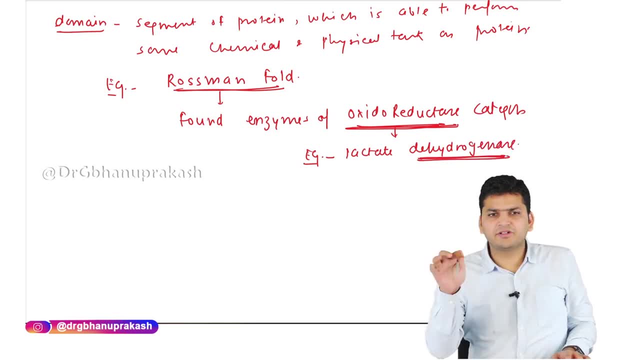 Lactate dehydrogenase, Lactate dehydrogenase- So Lactate dehydrogenase contains Rosman Fold and which is the example of domain. So now we are clear with the super second structure, we are clear with the domain, the. 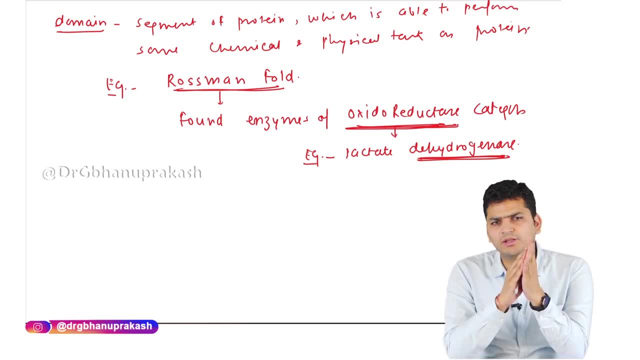 quaternary structure that is going to be more than one chain, but the bond that is going to be there in between is the non-covalent bond. So these are the points to be taken care of when we when it comes to the classification of protein that is based on the structure. 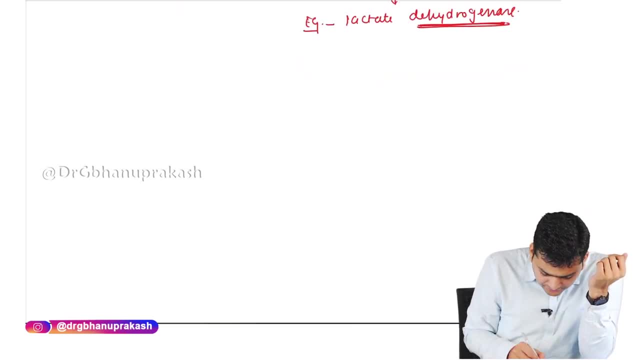 Now we are going to see the third type of classification of protein. that is based on the composition of protein. based on the composition of protein, See, when we want to divide the categories, we can easily say that there can be two types of protein. One is called as the we can say the unconjugated proteins. 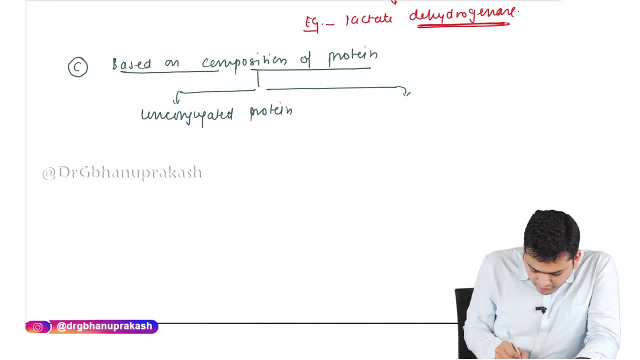 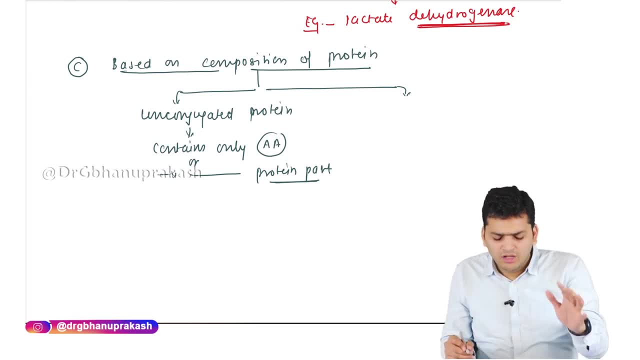 nothing else apart from that that is called as the unconjugated protein or a simple protein, Whereas something- then they say something- called as the conjugated protein. Now, what is conjugated protein? It is very easy to understand that there is going to be a protein part that is going 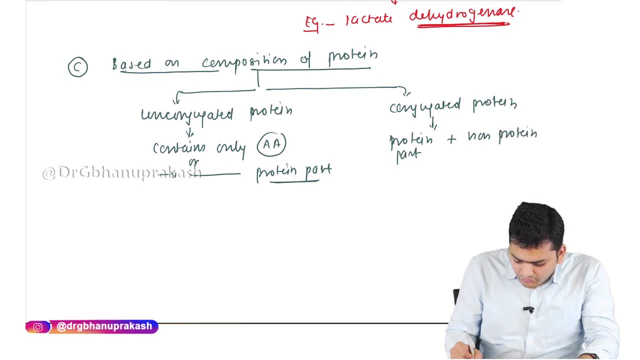 to be added with a non-protein part. If you add anything extra apart from the protein, that will be referred as the conjugated protein. So in unconjugated it is only the protein part that is going to be there in the unconjugated. 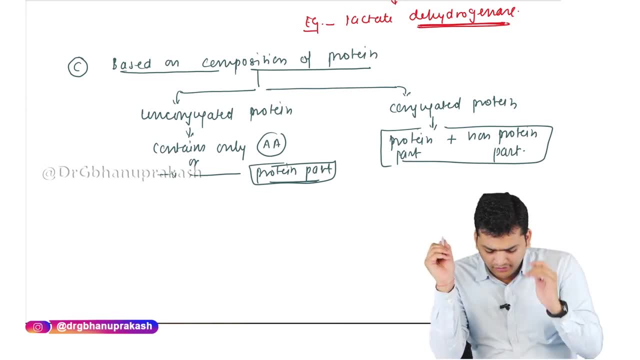 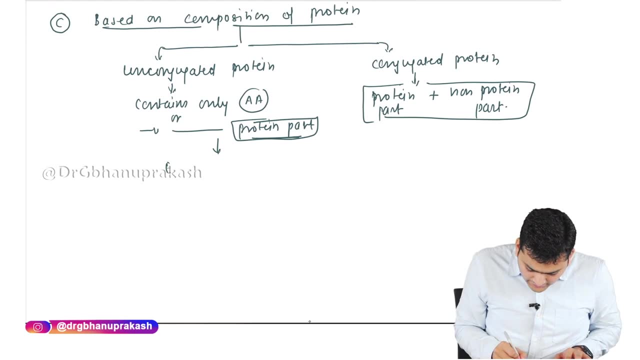 one and in the conjugated one you will have the protein part as well as the non-protein part. So, when it comes to the example, when it comes to the example of the unconjugated or a simple protein, the example of unconjugated one is the albumin. When it comes to the conjugated protein, the examples are, say, for example, glycoprotein, glycoprotein. Now, what is the meaning of glycoprotein? Glycoprotein means there is going to be protein. along with that, there is going to be glycoprotein. 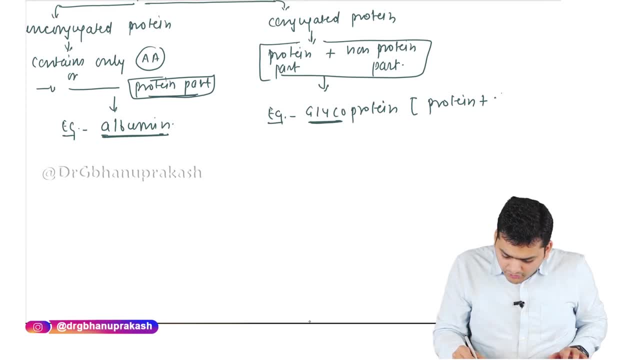 glycomin, the carbohydrate, and the particular carbohydrate that we are talking about here is the oligosaccharides- oligosaccharides- So if you take oligosaccharides type of carbohydrate, You add with a protein. the example that you are going to get is called as glycoprotein. 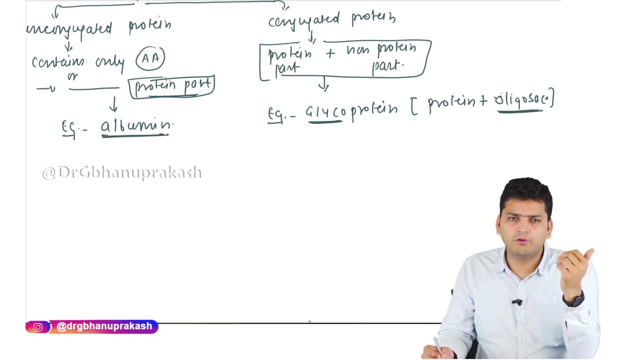 So they ask that: which proteins are found in the glycoprotein form? right, what are the examples of glycoprotein we have. the examples of glycoprotein that we have is blood group antigen, blood group antigen, blood group antigen, that is the A antigen or the B antigen. they what is the structure of them? they are the glycoproteins. they are the glycoproteins. One more example: What we can add is immunoglobulin. immunoglobulin, that is the antibody, that is also a glycoprotein. So these are the examples of the conjugated protein, the first example that we have discussed. 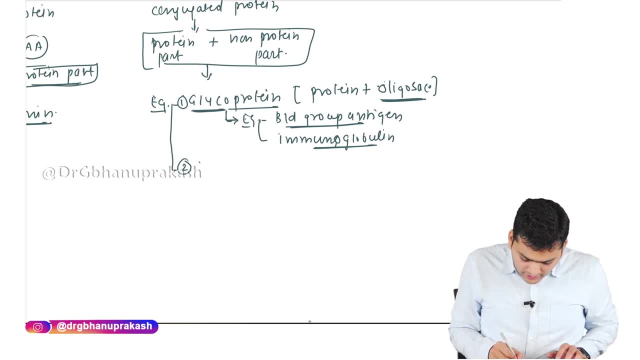 is the glycoprotein. Let's add one more example that is called as lipoprotein. Now this time the word itself is very clear, so we can say there is going to be protein and the known protein part that is going to be. there will be a lipid that is going to. 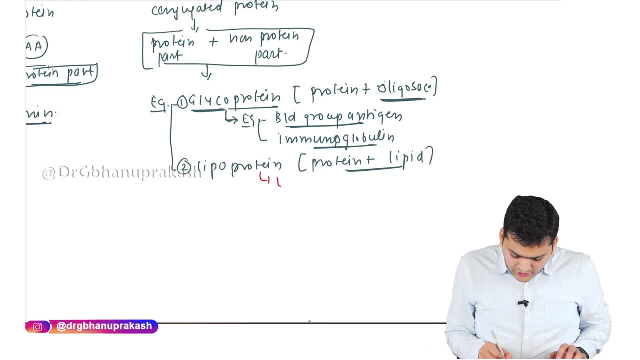 be a lipid, So that will be called as lipoprotein. So what are the various lipoprotein? that we know is the high density lipoprotein, HDL, the LDL, the VLDL. they are the. they are the example of the lipoproteins. 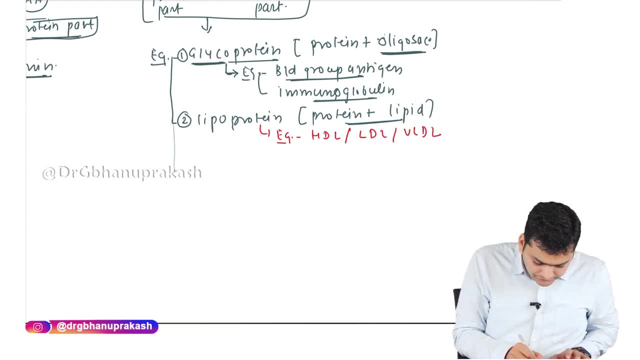 Then we can add one more example of the conjugated protein that is called as nucleoprotein- nucleoprotein. Now, what is nucleoprotein is? obviously there is going to be the protein part and along with that, if you add the nucleic acid, 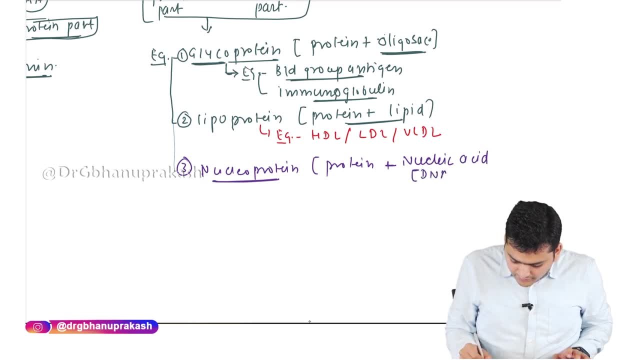 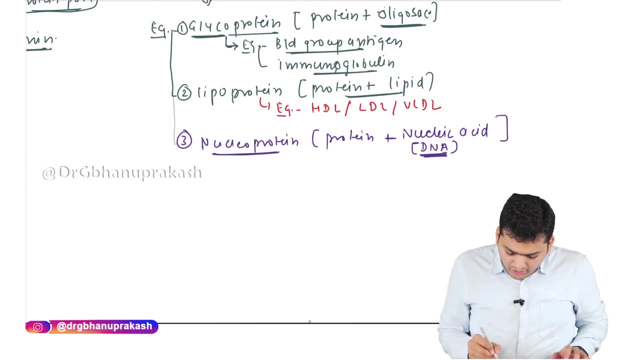 So nucleic acid means DNA or the RNA, But we primarily talk about the DNA. so if you take the protein along with that, if you add the DNA, that is called a nucleoprotein. the protein that we are talking about here is the histone. 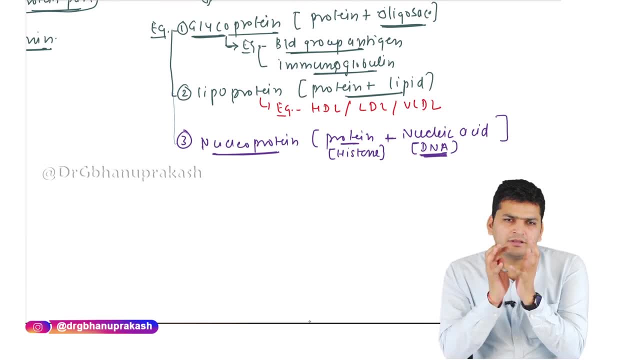 So if you take the histone molecule, you add with the DNA, that entire unit is called is the nucleoprotein. So what is nucleoprotein is basically histone with the DNA, histone with the DNA. what is lipoprotein is the lipid with the protein. what is glycoprotein is the protein with the 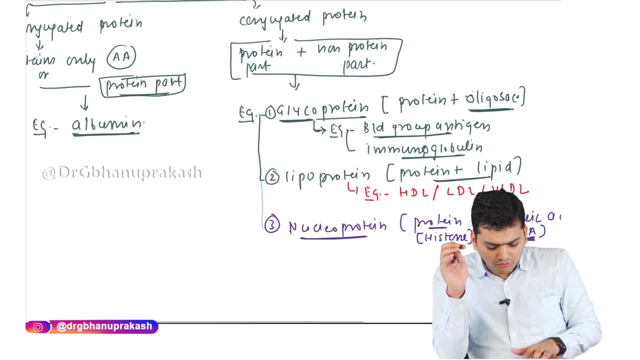 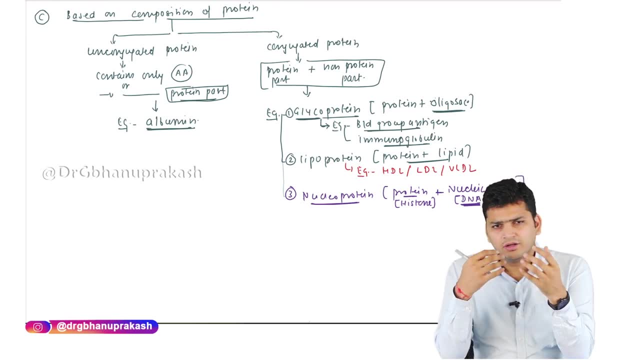 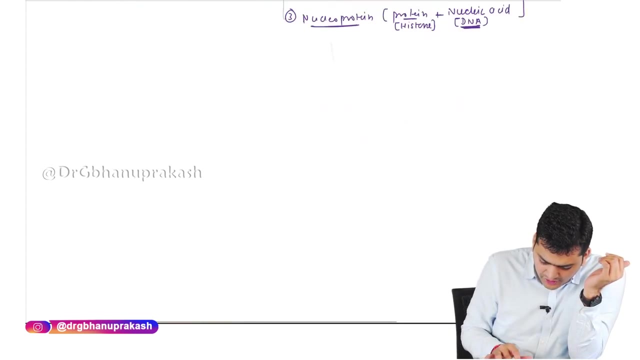 olycocytorynase. Right, Ok, so these are the examples of the conjugated protein. so this is the second. this is the third type of classification that we have discussed that is based on the, the composition we can say is the conjugated or the unconjugated type. now, the last type of classification of protein, that we can do is based on the shape of the protein, based on shape of protein. now, when we classify the protein based on the shape, i can say there are two types. there are two types: one is the fibrous protein- fibrous protein- and the second is the globular protein. 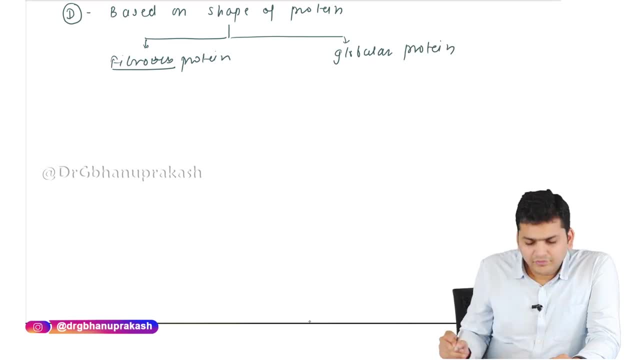 fibrous means there are going to be fibers. globular means there are going to be the spherical molecules are going to be there. so fibrous, the shape is elongated, like shape. they are going to have elongated fiber shape, whereas globular they are going to have a spherical shape, spherical shape, spherical shape. so the fibrous molecules and 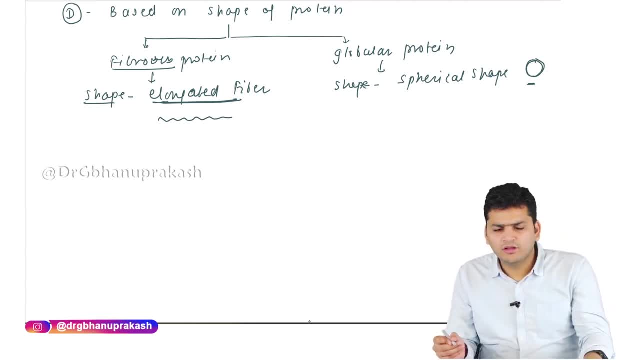 the spherical molecules. so there are two types of protein based on the based on the shape. now, what is the use of knowing this concept? see, the fibers are used to make the shape of the protein, based on the shape of the protein. then first two fibers are the inner solid. first two are the insoluble fiber. 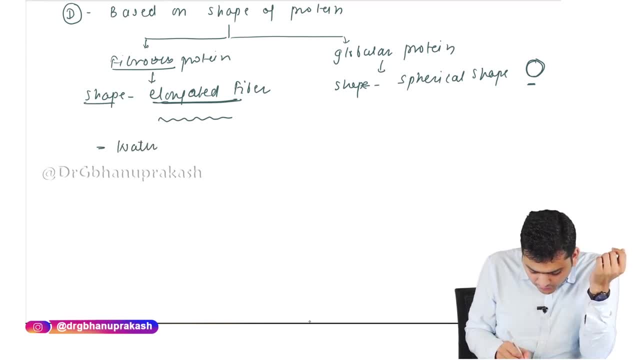 the physical elements are the insoluble, but they mix with each other and their formation is released. EUarea they get per corruption in volume of the freelance nation. all those are water insoluble proteins and once it makes the shape the first fiber, they are used because fibers are water insoluble where the spherical molecules are water soluble. 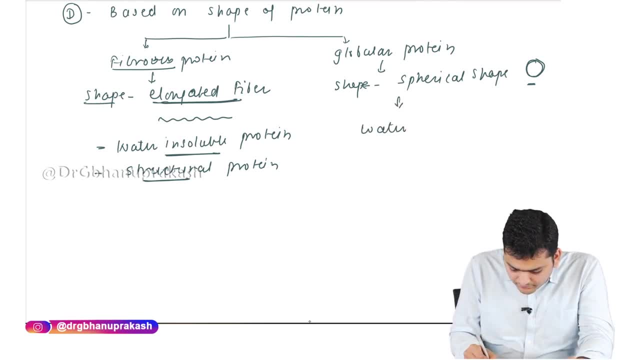 so i can say the fibrous are water insoluble proteins. once i am saying that they are water insoluble so we can make latest body structures from them. so they are basically the really are soluble. they are water soluble. so basically they are going to do all the dynamic functions. 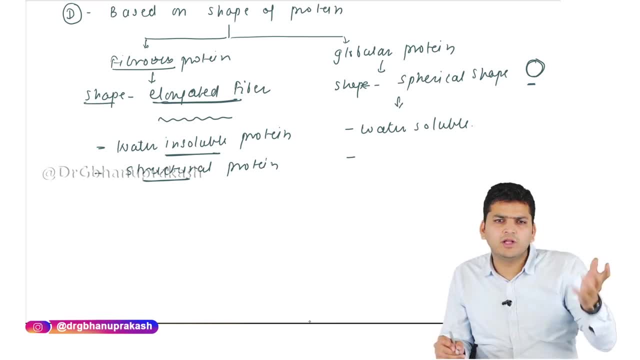 means they will move from one place to another in the body very easily and will do the dynamic functions. so i can say they have the dynamic functions, they will do the dynamic functions. when it comes to the example, the fibrous protein. example is collagen, elastin, fibrillin- these 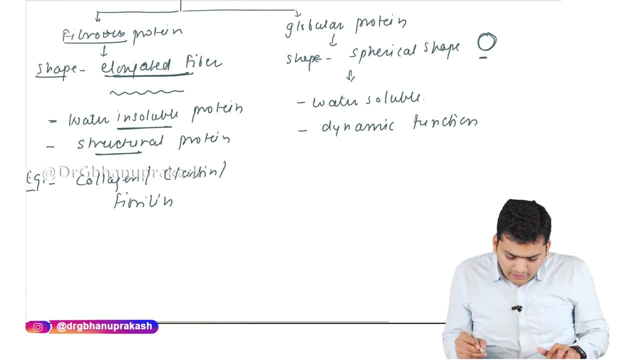 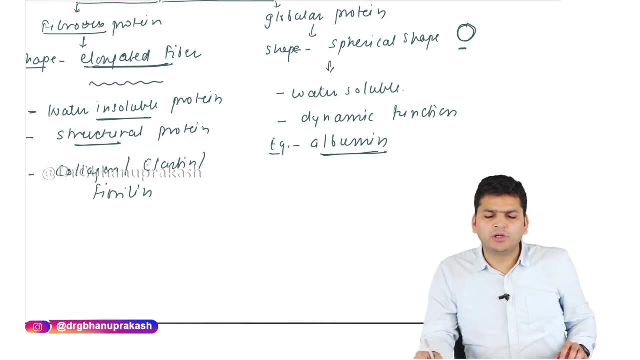 are the example of the fibrous protein. when it comes to the example of the globular shape protein, let me say, for example, albumin is a spherical protein, it's a globular protein. so, based on shape, we can see that protein can be divided into two category. one is the 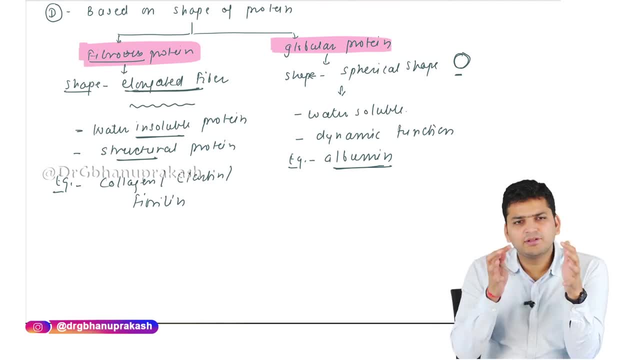 fibrous and another is the globular protein. the fibrous is going to be the having a elongated fiber-like shape that is going to be in the most of the structure of the body right say, for example, the collagen, the elastin and the fibrillin. and when it comes to the globular,